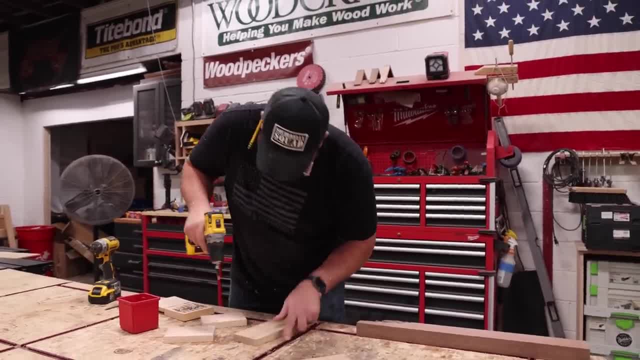 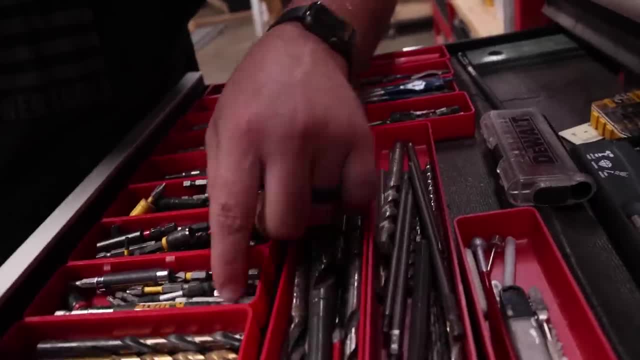 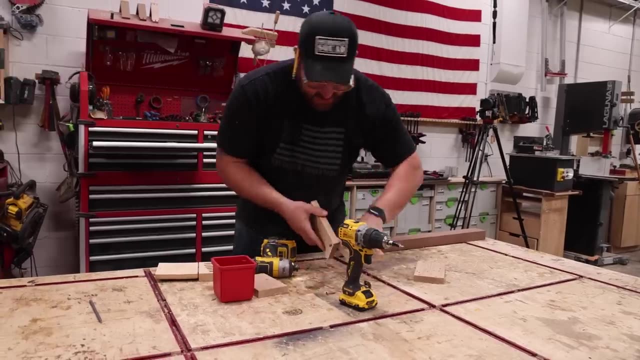 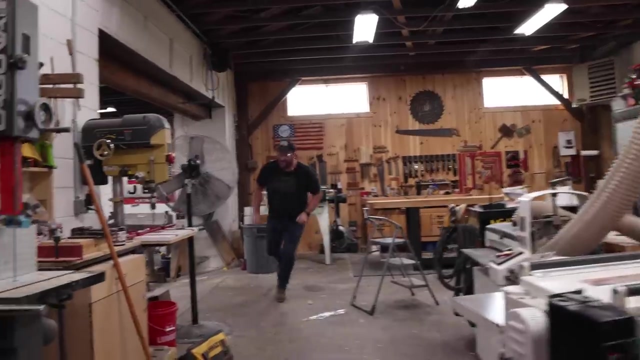 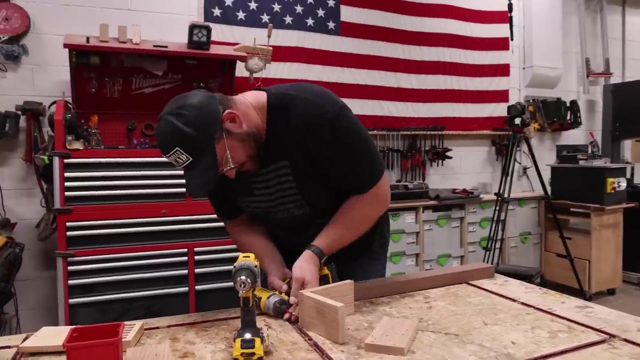 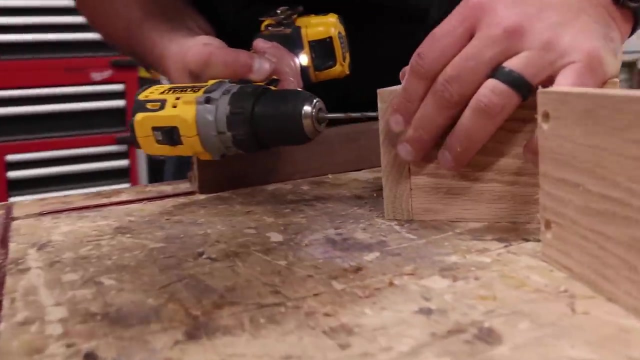 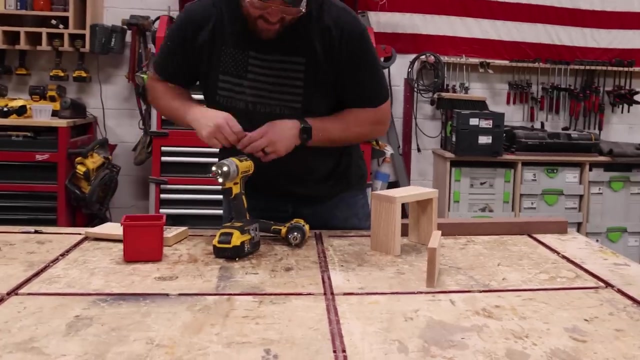 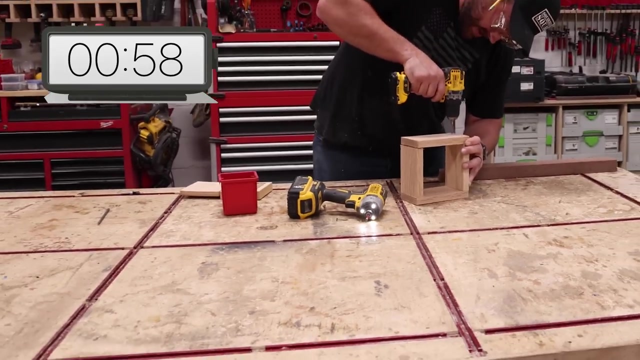 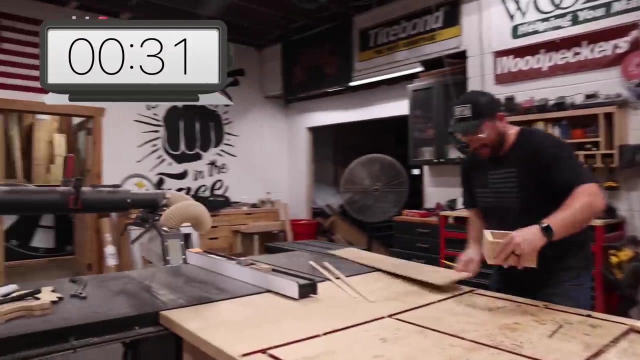 As it looks so easy on television. Yeah, I need a bit for this, The only screws we have, and that'll work. not enough for me. two minutes 30 seconds, Oh, Oh, Make it. Oh, my goodness, I'm sure that Garmin is perfect. Thirty-three seconds training. 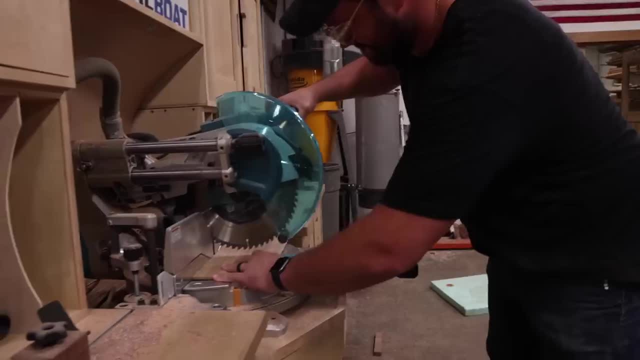 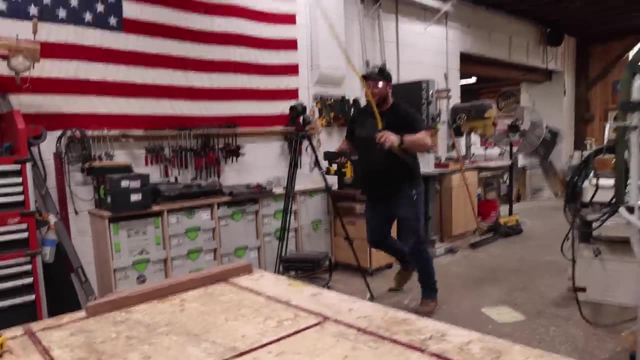 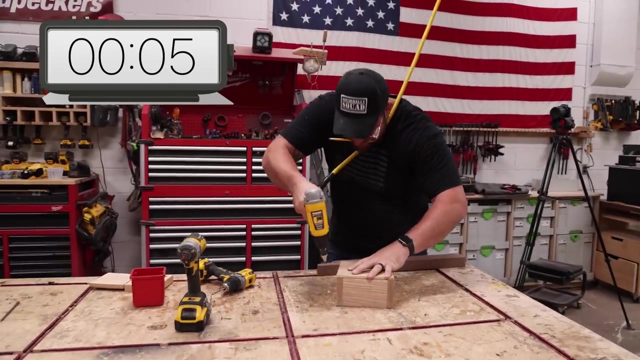 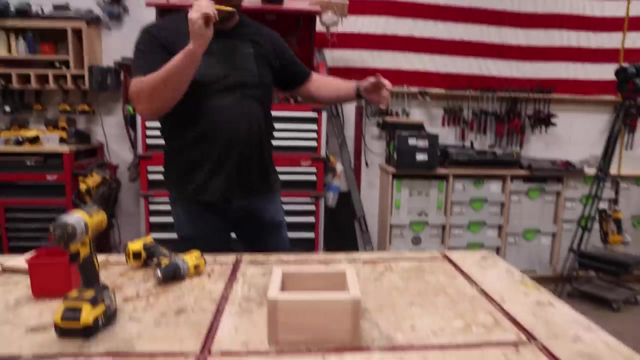 15 seconds. I don't even know what the hell's in here. 10,, 9,, 8,, 7, 6, 5, 4,, 3, 2, 1,. game over Box. 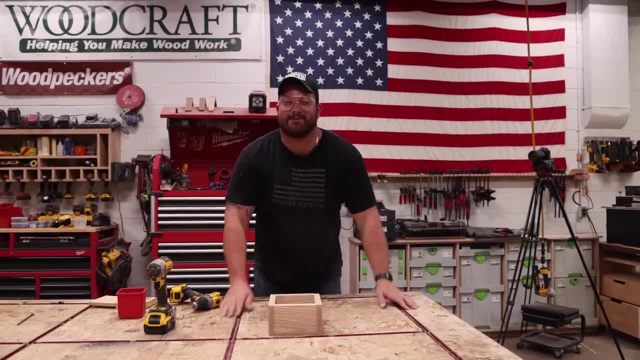 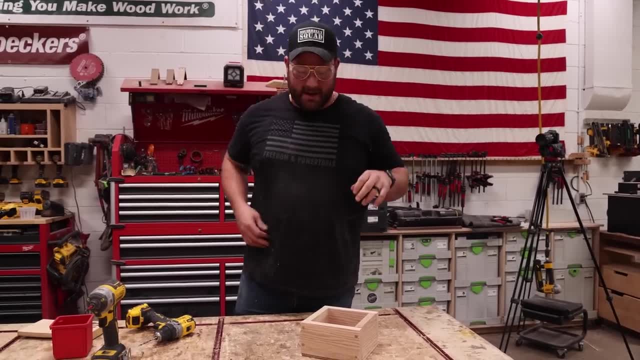 Wow, That was awful Shocked. I am sweating. I can't believe. something looks like a box. You know, what's funny is I really underestimated how much time things take- and I always do that- but I thought I was going to have time to put some like nice plugs on this and stuff. 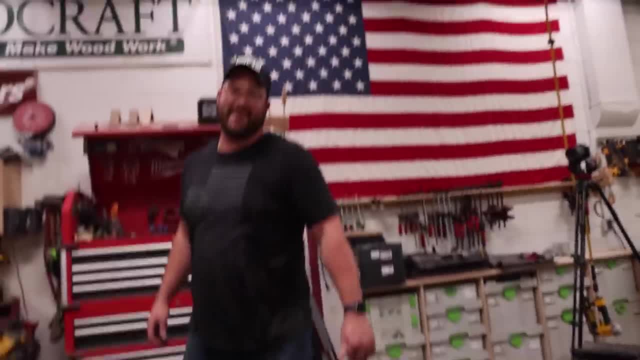 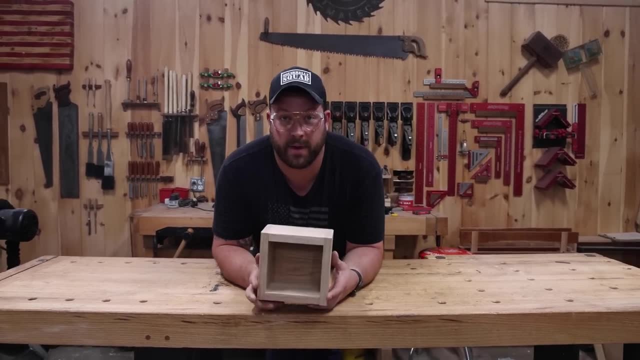 Not at all. I need a break, A cup of water- Yes, Let's hydrate, All right. So after I caught my breath looking at this thing, it looks like a five minute box. You definitely clean it up a little bit with some sanding, some finish, but I cannot believe. 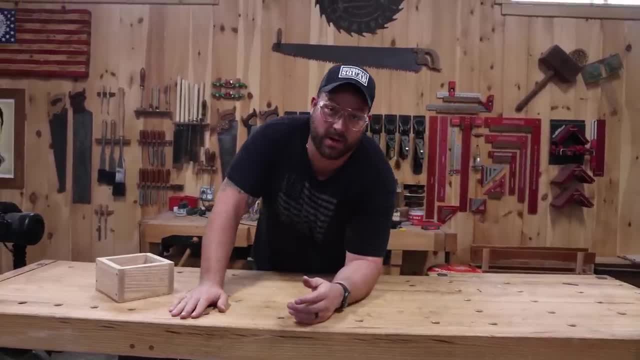 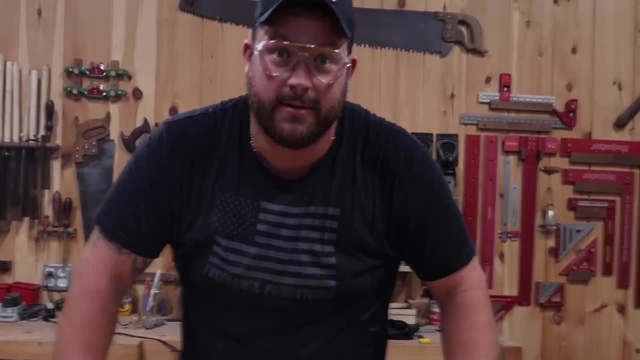 how fast that five minutes went. The next one should be pretty interesting. We're going to do a cherry wood box with splines. I'm going to out-build the spline jig in the 50 minutes, so let's head back over to the 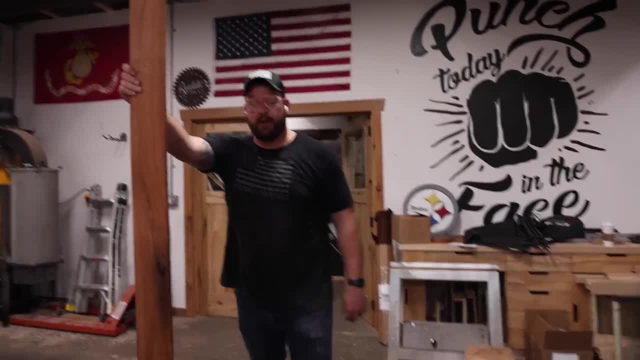 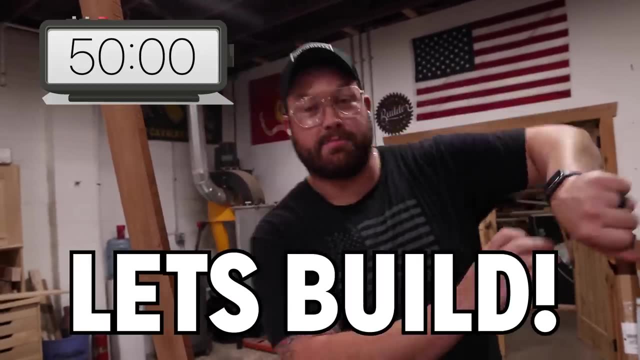 table saw. So I got this single board of cherry and I got my stopwatch. Sam's got his set up, ready to roll. Three, two, one, Let's build. First thing I'm going to do is make the panel for the bottom. 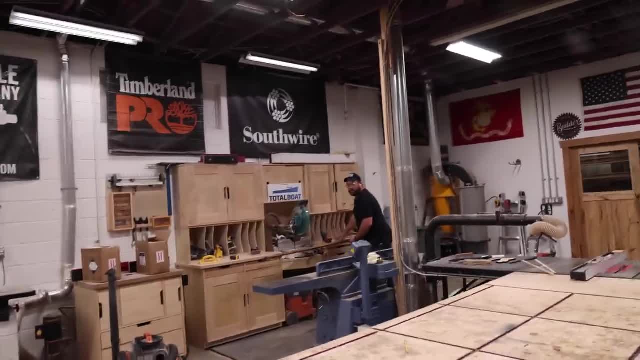 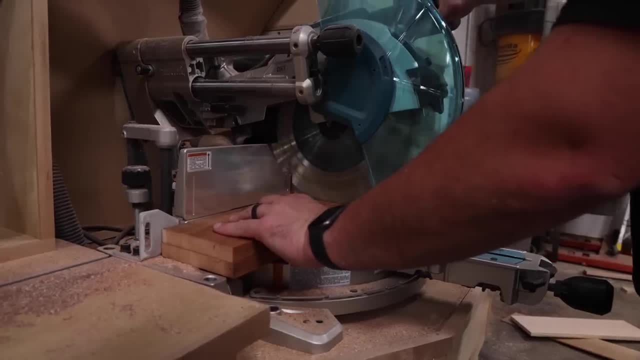 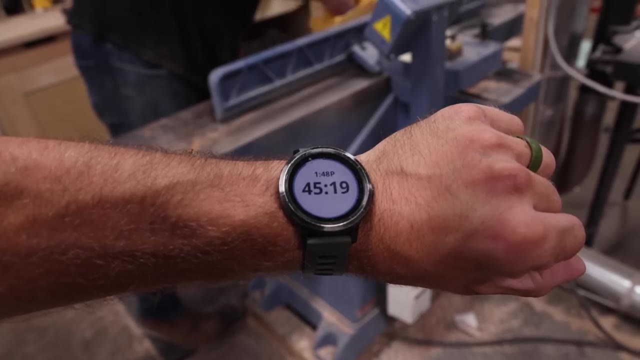 I'm not going to cheat. this time I'm going to use glue up. I'm not going to cheat. this time I'm going to use glue up. I'm going to use glue up. I'm going to use glue up. What happened to my joiner? 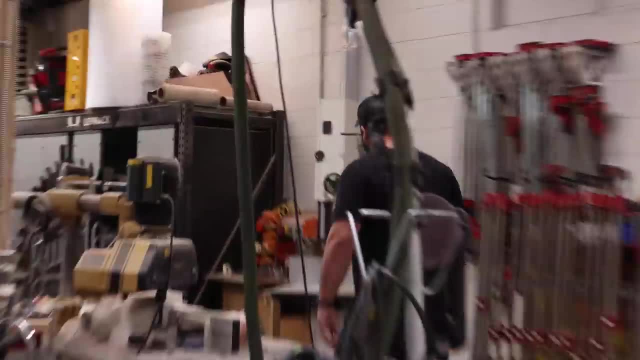 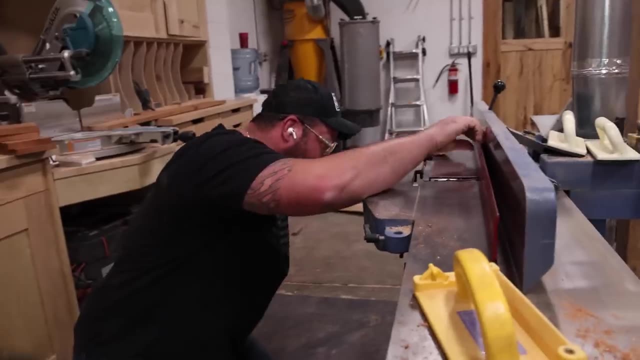 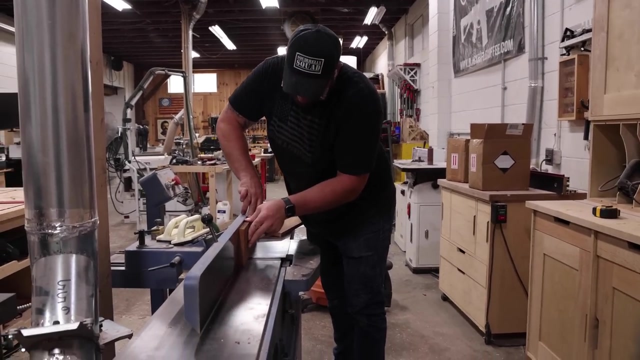 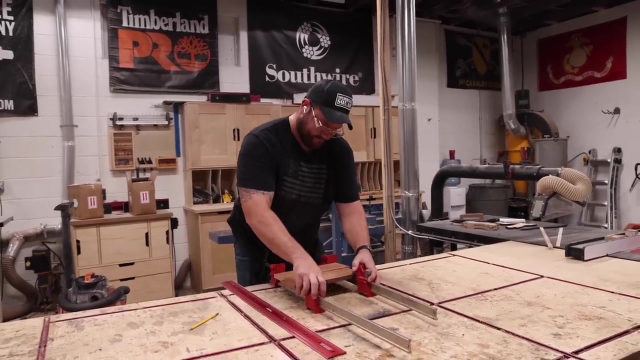 What's wrong with that? See that? That's not how it's supposed to be. We're going to use a fast drying glue. We have 42 minutes and 14 seconds left. That took 8 minutes. It should have taken 3.. 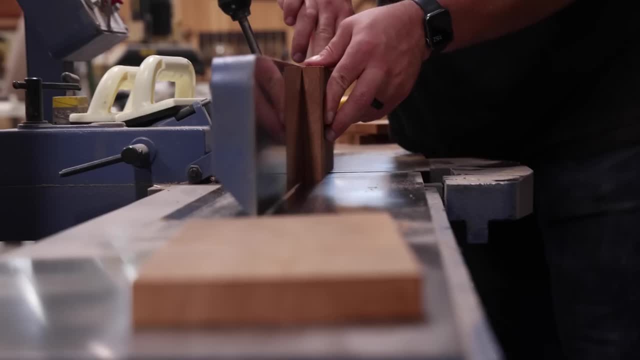 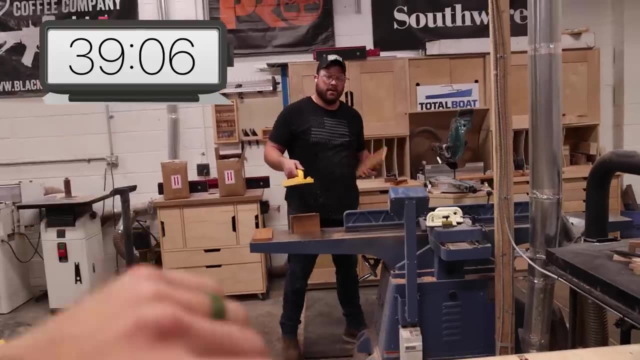 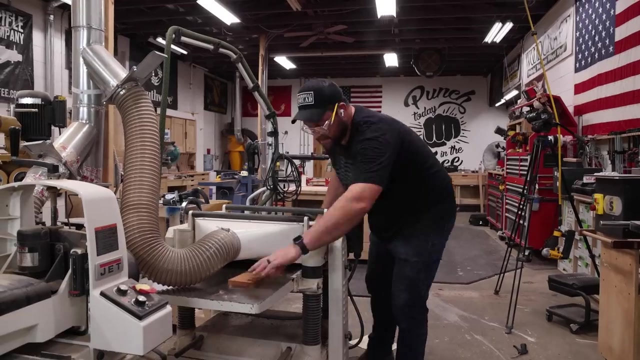 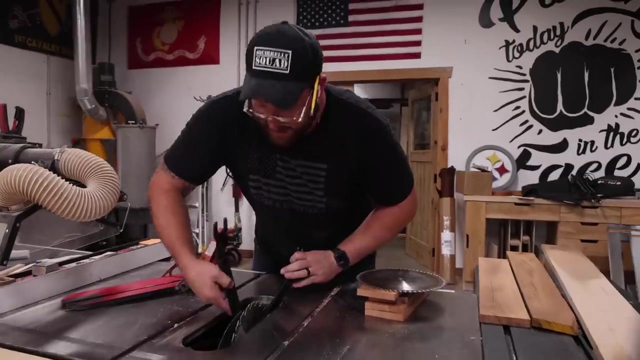 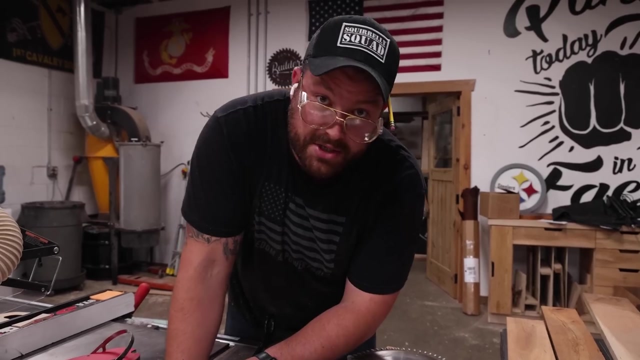 Here. our outfit table came out of whack 39 minutes Rip blade in here right now, which will make terrible tear out, But I can't. I'm going to sacrifice that on my biters. Fortunately, a couple of years ago I built a sled for the type of box that we're building. 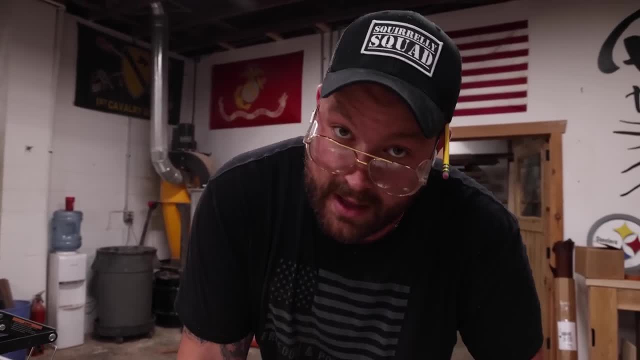 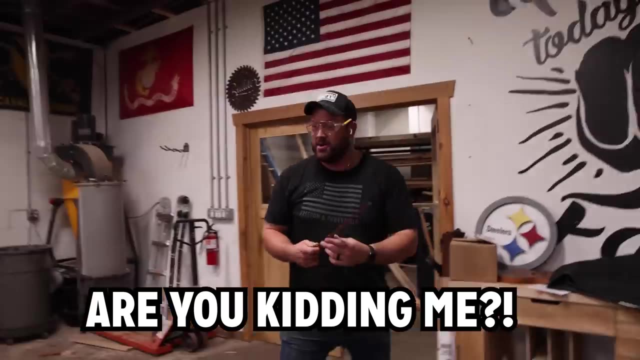 You should be able to just chuck that on here, Adjust the blade, There we go. It's going to get really close to where I'm trying to build. Are you kidding me? All those screws? None of them are ever going to. 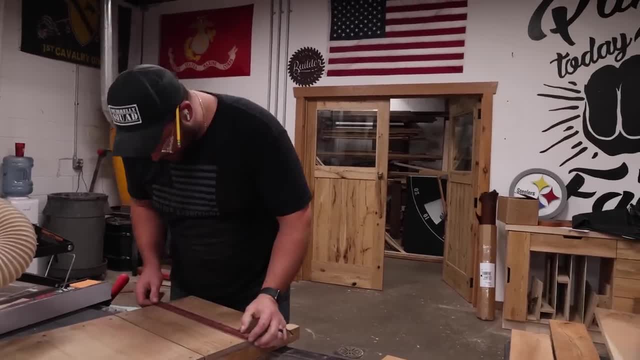 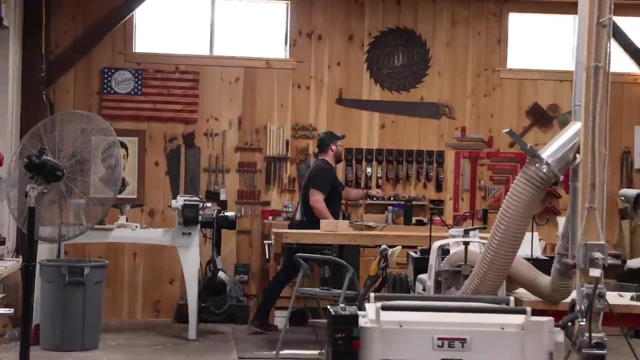 I've had this thing for six years. I blame Jordan. Dammit Jordan. I'm going to take a little less. Sam's help, Is that going to be against, Or do it? I have lots of plan and this is going. Let's go. 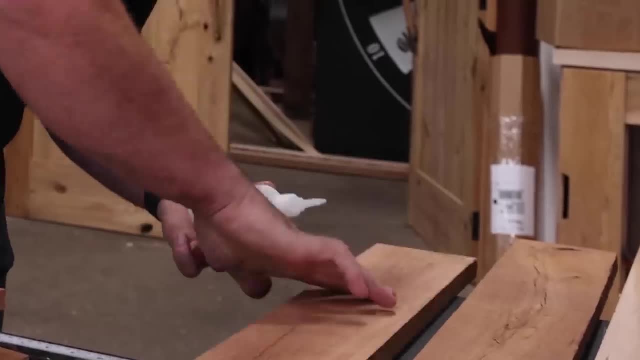 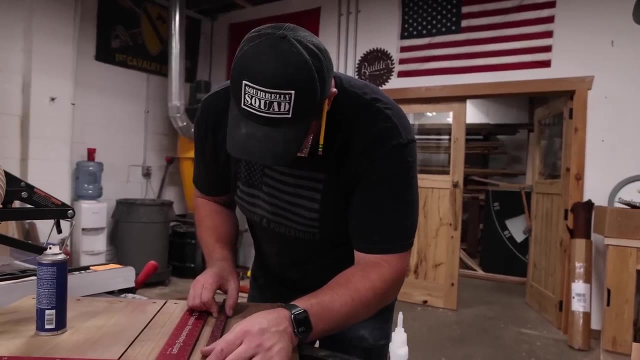 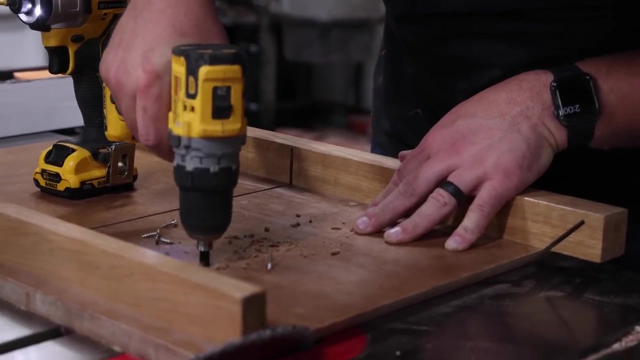 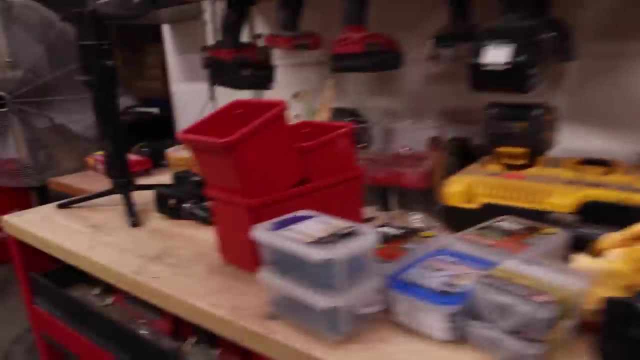 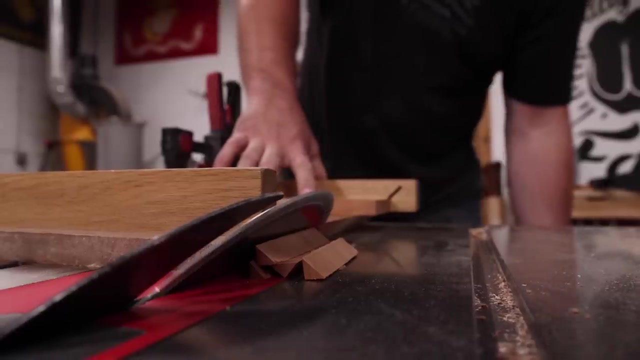 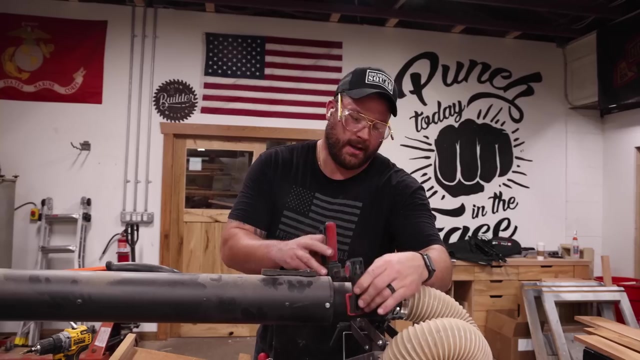 What do we, what do we like to say around here? Sam, slow, smooth, smooth, fast, 34 minutes. They couldn't have been in a dumber place. I can now put that ripping blade back in and rip the panel bottom. 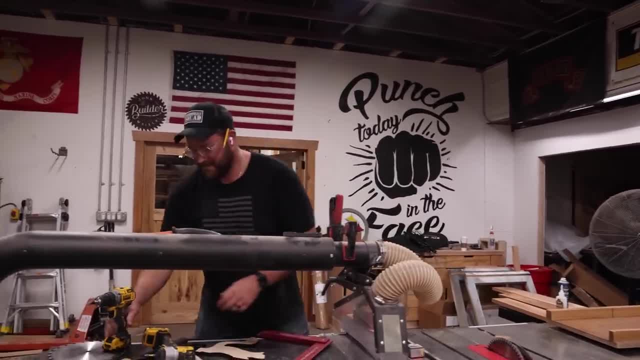 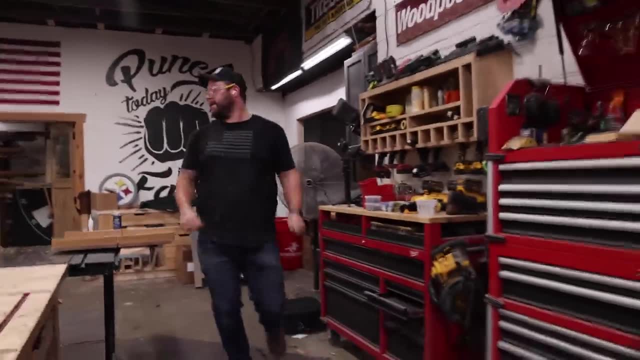 High speed woodworking Wouldn't build for this. I can't believe it's already been 20 minutes, Like I feel like I did nothing. All right, So I need to get this panel on the bottom cut to size. I'm just praying it's dry. 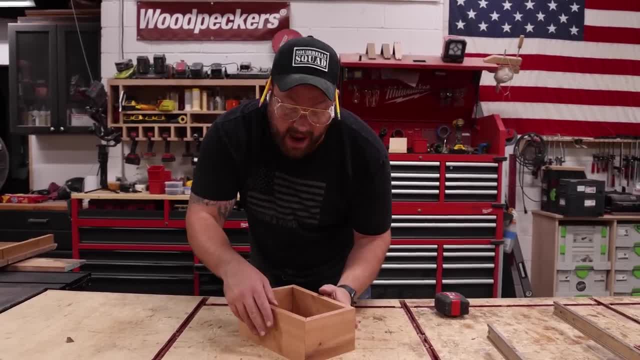 The only thing Sam's helping me with on this entire build is the dust collector. I'd have that thing running the full time, but you can't hear me then, So Sam's being an adult about it and turning that thing on and off. 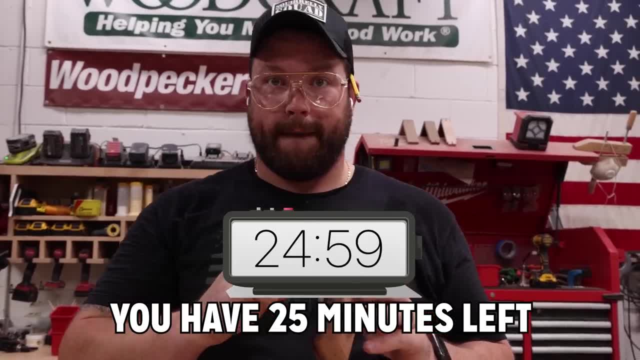 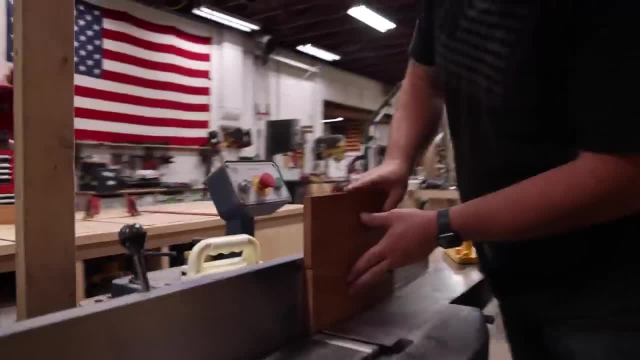 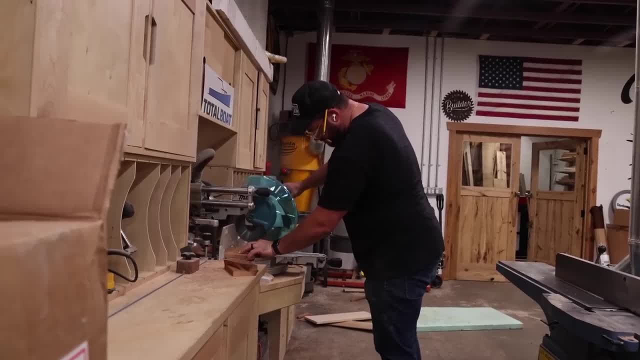 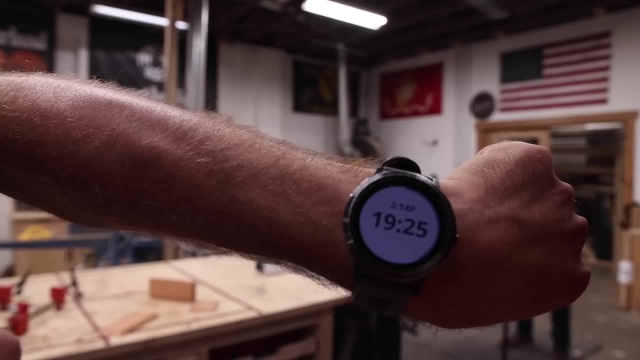 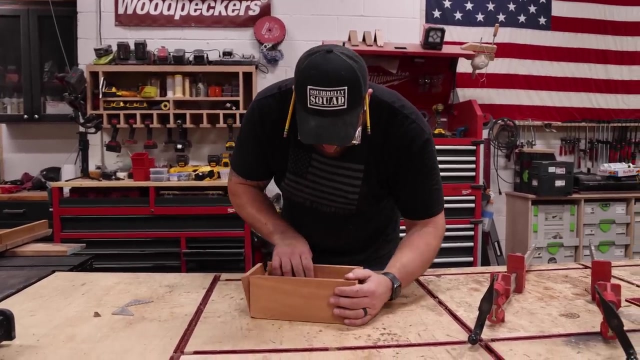 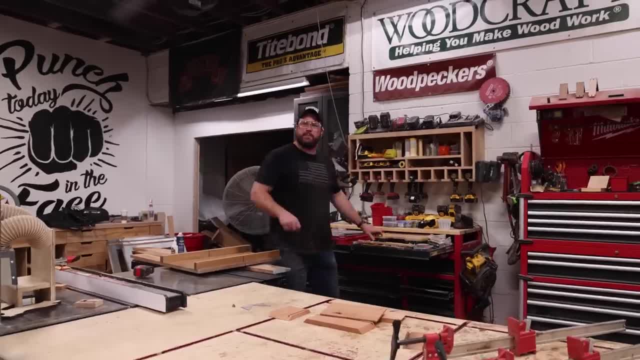 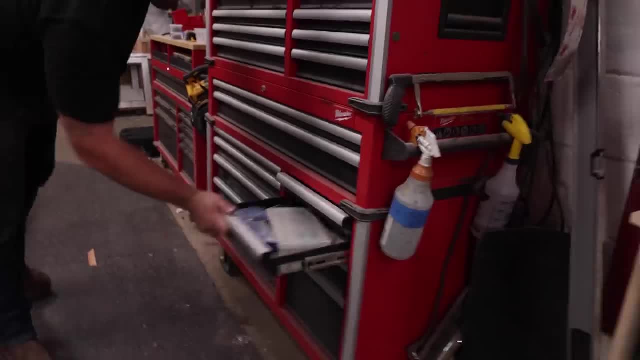 Yup, Yup. So that's a lot better than the product right now, that's a lot better than it looks like And since it's a wire for this, Next, My spinal cord. It hurts. I don't know what that means. 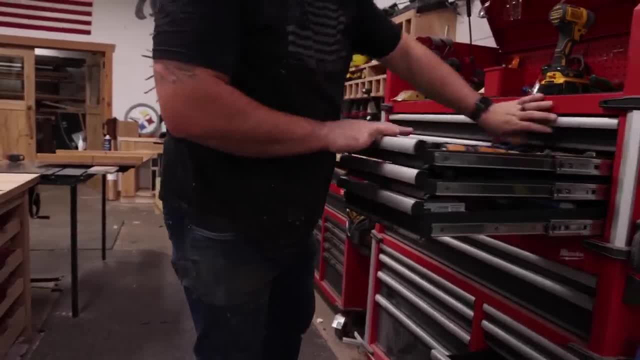 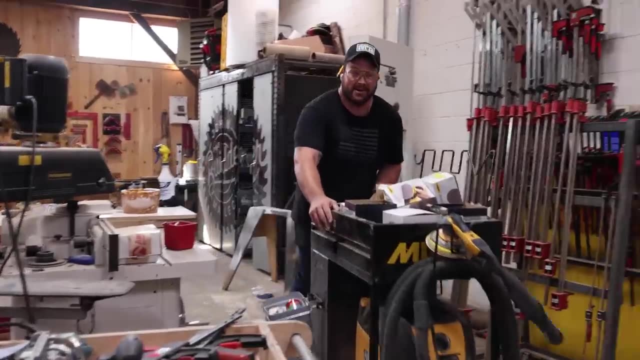 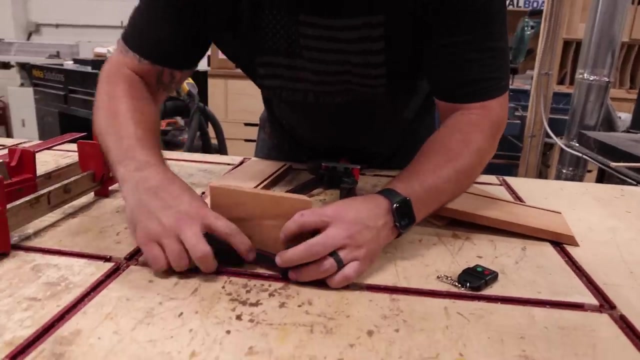 To keep me that too short. it sure did. Damn it, Spaceballs. I'm joking, this is funnys Bye. We got a slim chance of hell here, Sam. A slim chance of hell. I'm gonna go ahead and forget, all right. 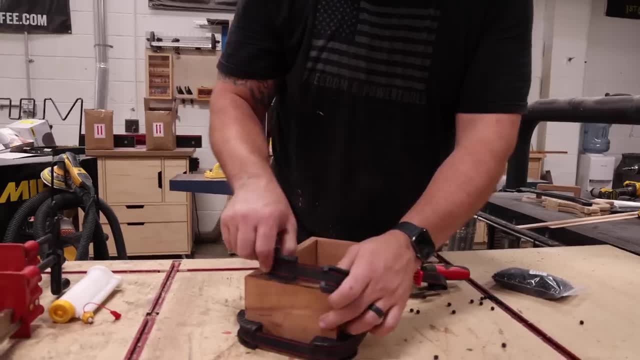 Pretty sure they claim this dries in 10 minutes. We gonna find out today. How much time do I got Sam. 12 minutes 10 seconds We're I'm. I like how this turned into like three cool ways. 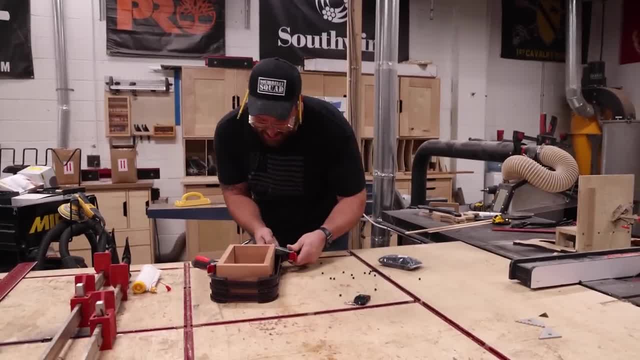 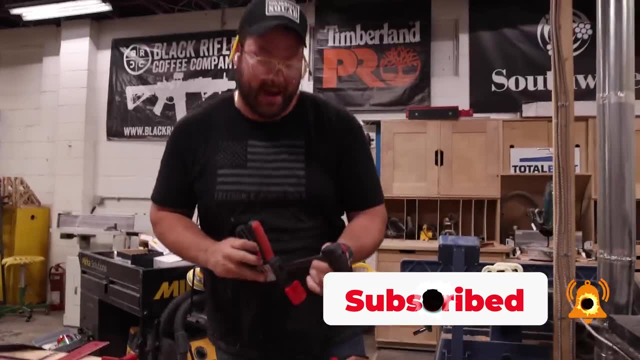 to do something in a short period of time To like me being absolutely dripping sweat getting my ass kicked. I guess that's more entertaining. I'll do it for the peoples. I thought this. I had plenty of time to do this one. 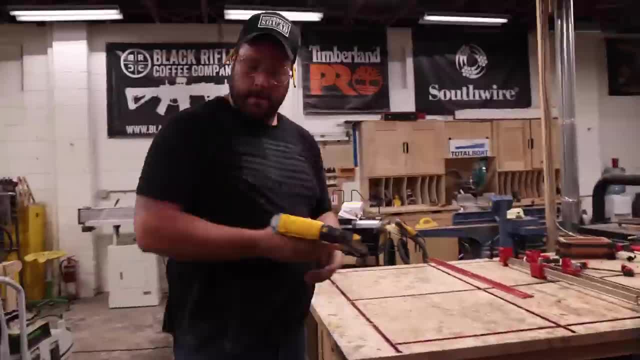 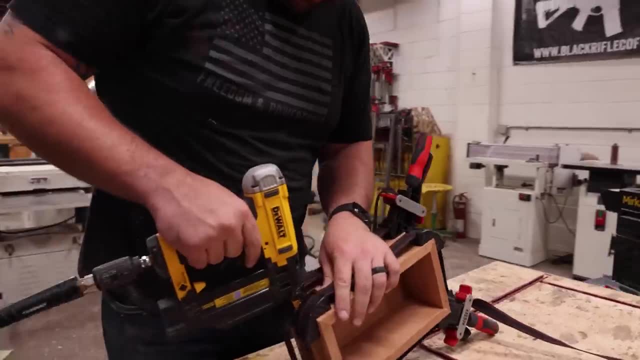 I know what I'm gonna do: Pivot, I'm pivoting, Sam Cause I wanna get the splines in. What I'm gonna do is throw some pin nails That'll be hard to see. This was such a stupid idea. 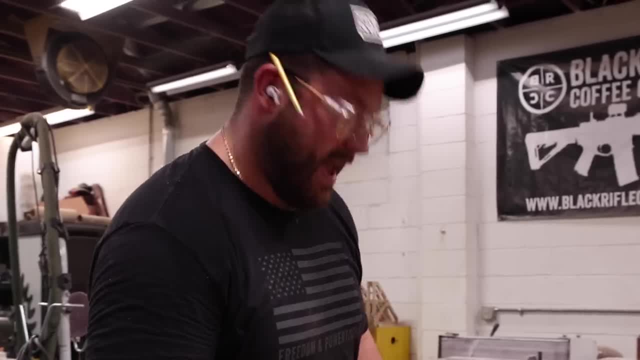 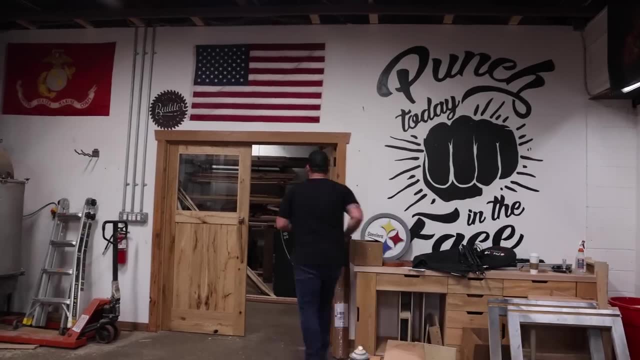 I've nailed this into it. great On the cooking one: they lie It says the time, but then that's only the time that it takes to cook, Not prep. you bastards. I need a fricking material to spline. 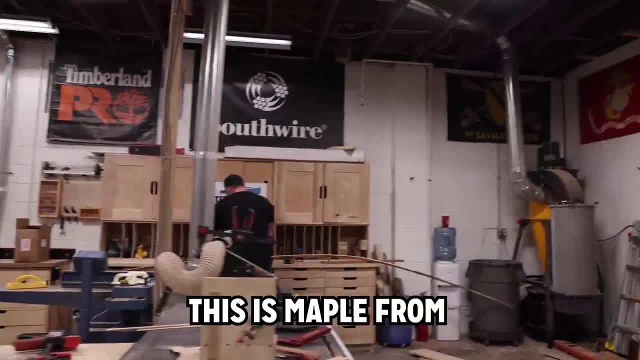 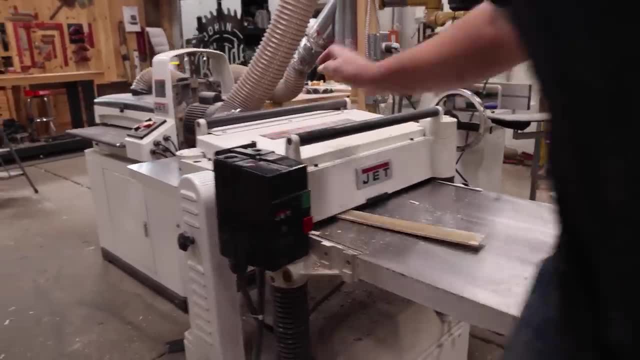 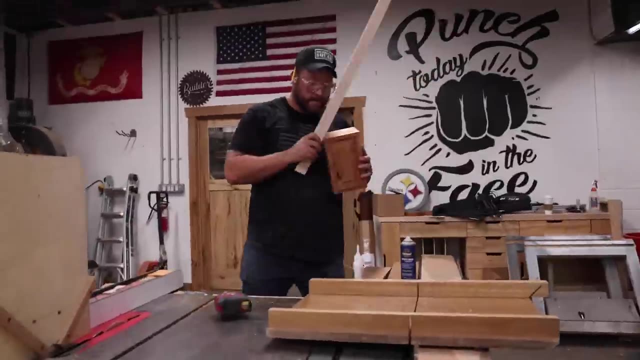 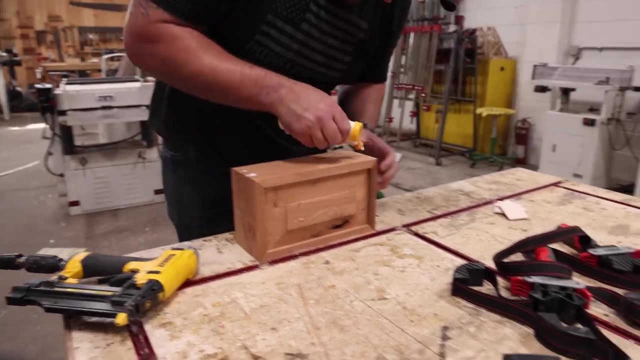 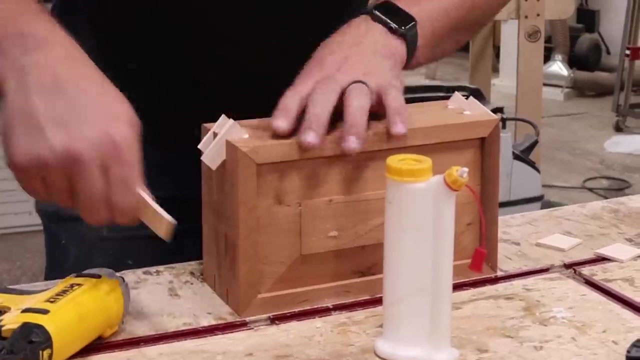 Ah No, Is that plywood? This is maple from something Man. that's a first Six minutes 30 seconds. I'm going to ask again Who, according to my idea, was this Fine huh, Five minutes. Usually I do this by hand, but 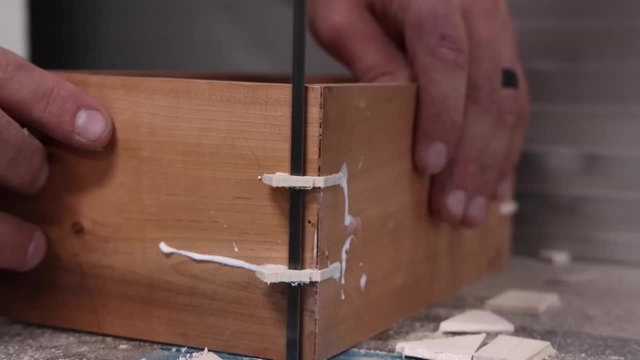 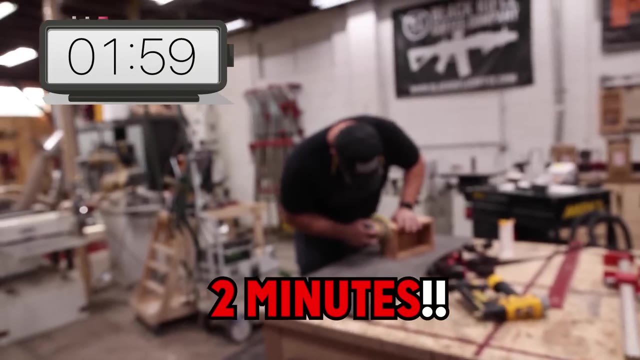 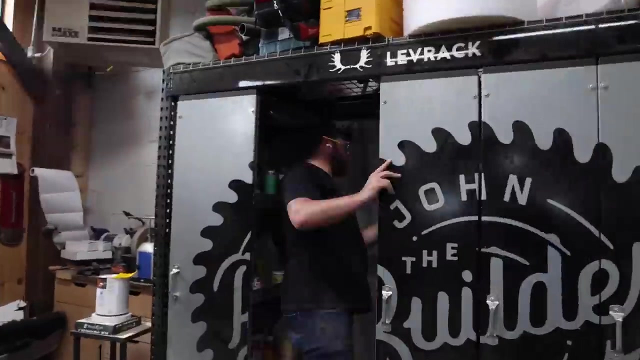 I ain't got time for this sh****. Hey, nobody got time for that. See there, Look at that. minus Uh-huh. You guys want it to be kind of out like this. Yeah, Bonnie, Just like that, You made 7 minutes like that. 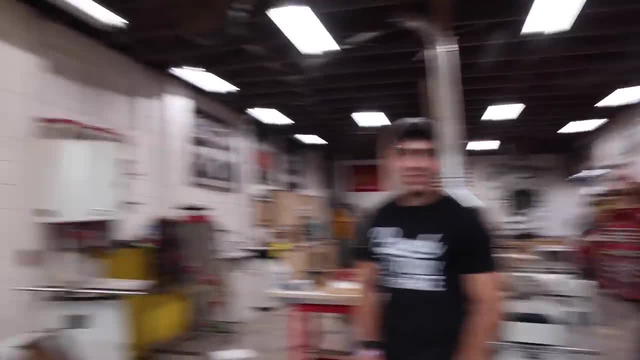 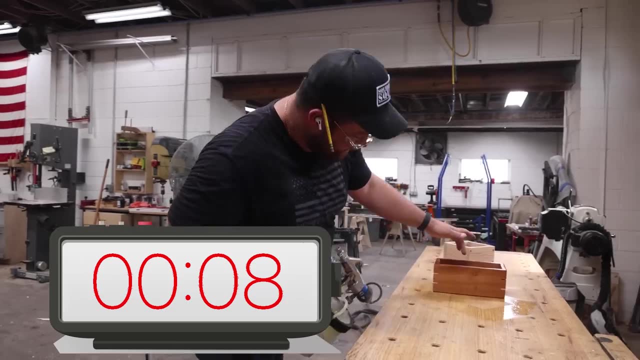 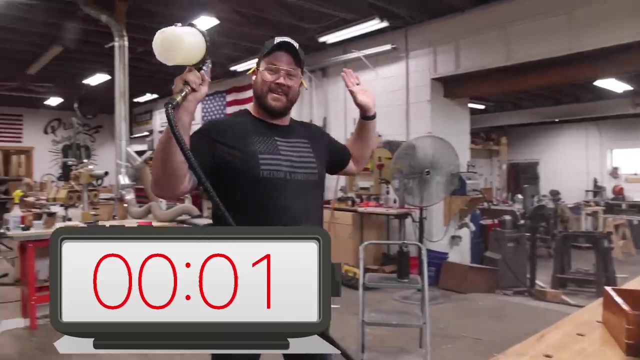 30 seconds Spray finish. We don't have anything clear-fitted. huh, ATLP may have something in it. Eight, seven, six, five, four, three, two, one and time. Oh, my goodness. Oh, that's the spline. 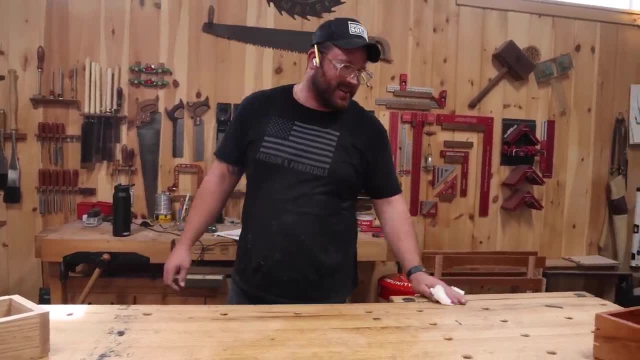 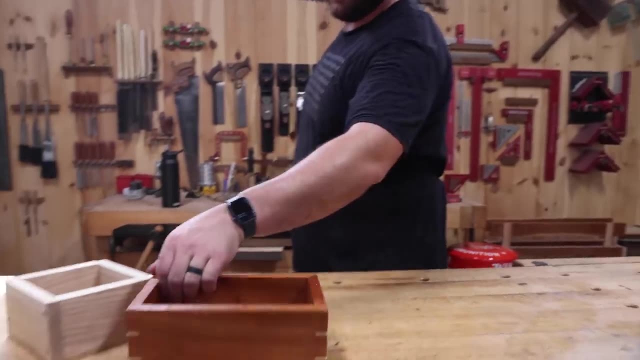 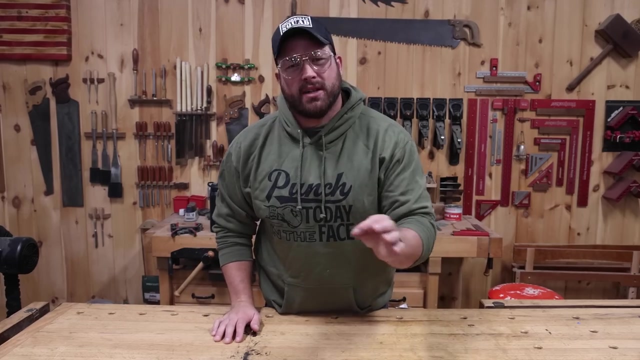 I can't breathe Mineral spirits. No, no, no, no, no. Your time's up. Hey friends, real fast. before I dive into the last box here, I want to take a second to thank the sponsor of the channel that we love the most. 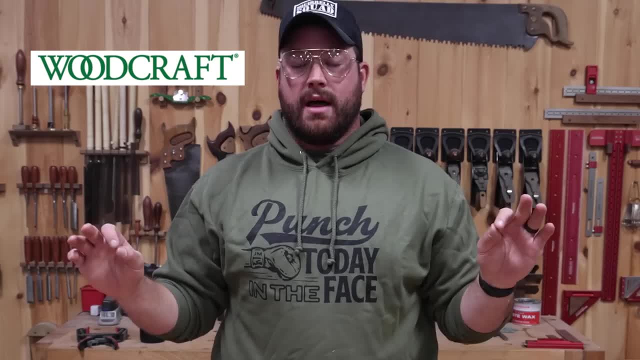 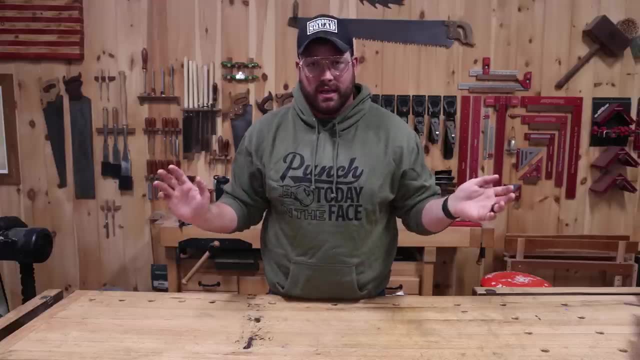 when it comes to woodworking, Woodcraft, If you guys aren't familiar, Woodcraft is bar none the best supplier and distributor of woodworking products in the world, in my opinion. They've got storefronts across the country, I think in like 74 different cities. 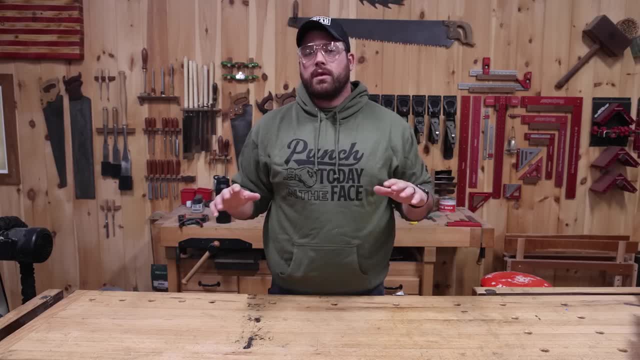 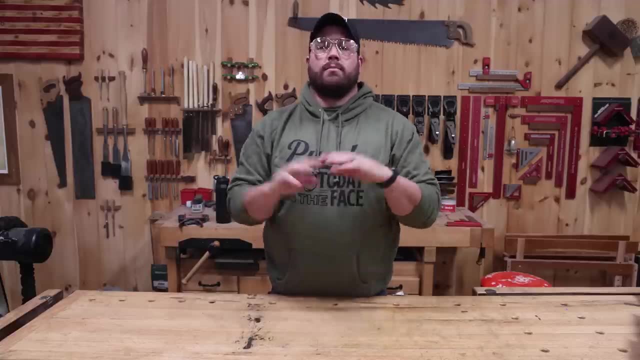 and as well as an incredible online store. If you're looking for anything woodworking, they're going to have it. Most of the stuff that you can see in my videos is available at Woodcraft. So find your local store. go online, be awesome. 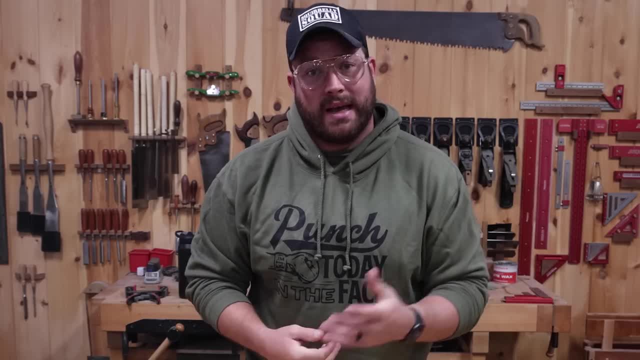 check out Woodcraft. Thank you, guys for supporting the channel these projects. Now let's see if I can get something done in five hours. All right, so for the five hour build we're going to do a lidded box. 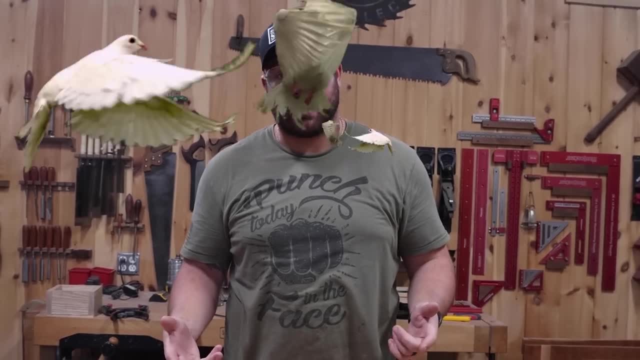 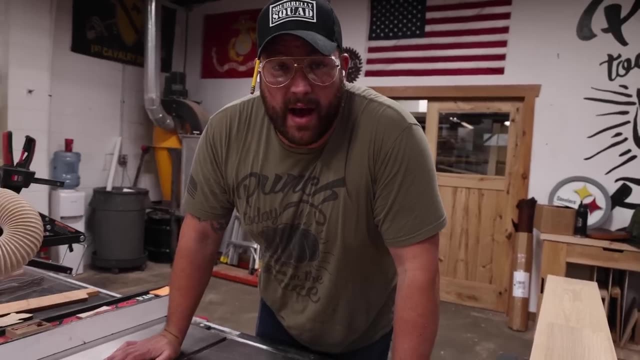 and I'm going to do a little bit of a detailed feature. We're going to do dovetails on that box, as well as multiple wood species. Things should get interesting on this one. Let's go rip some wood. So we've got five hours on the clock. 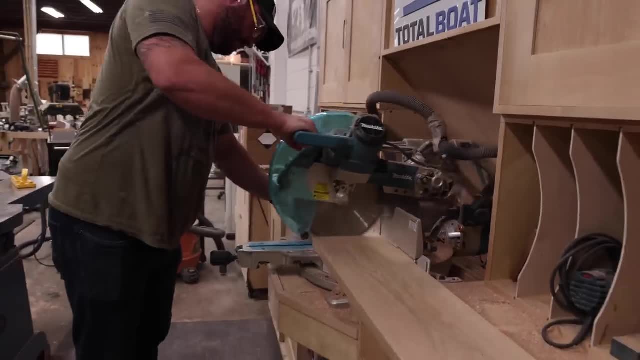 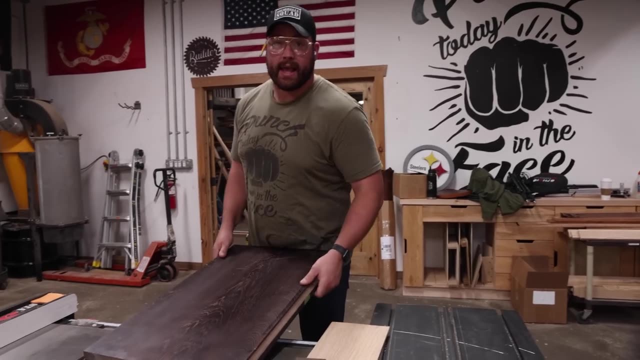 Let's get ripping. So I'm going to try to make this thing out of wenge and white oak. I've got some white oak that's raw, but this wenge here I have leftover from a project that a client sent back to me like six years ago. 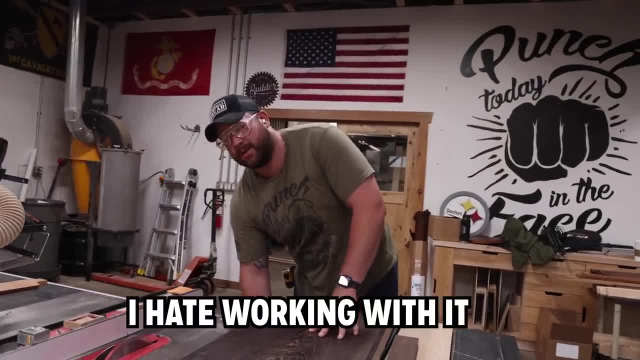 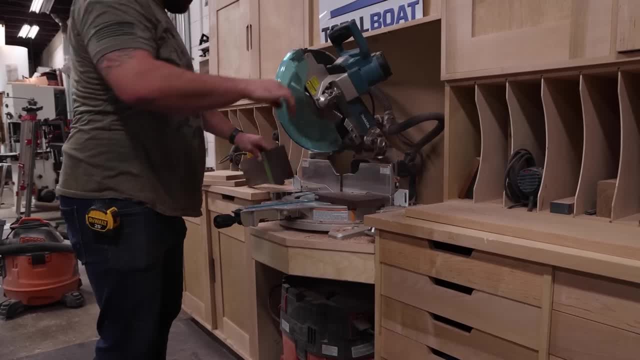 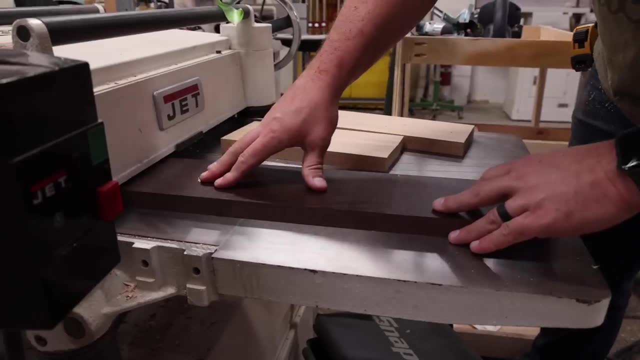 So I want to get that dark contrast. This stuff's super nasty and I hate working with it, But I'm going to try to get it done pretty well and hopefully I get some good edge. I've got a bit of Q-tip on the back here. 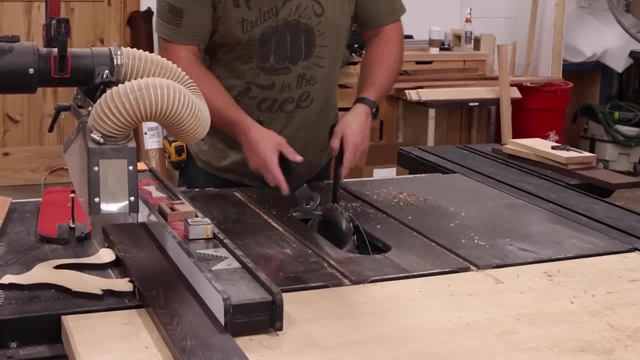 I'm going to try to make a better shape and I'm just going to start off with a little bit of wenge. We're here, We're going to have to go back and forth. If you give me time, I'm going to do it again. 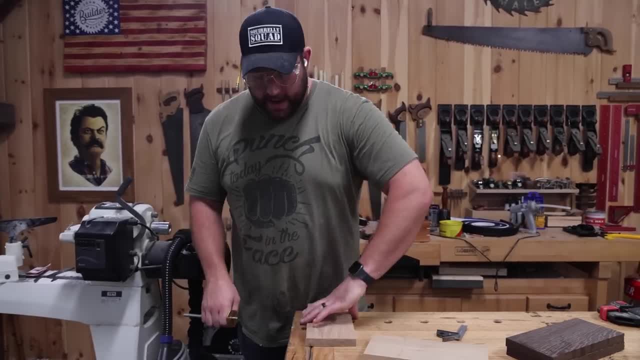 See if you can see that little thing there, See if you can cut off some of that. So I'm going to go ahead and give it a go. I'm just going to kind of cut around it and then I'm just going to pass it along. 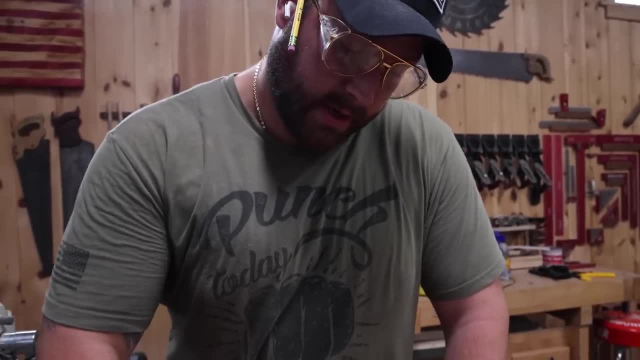 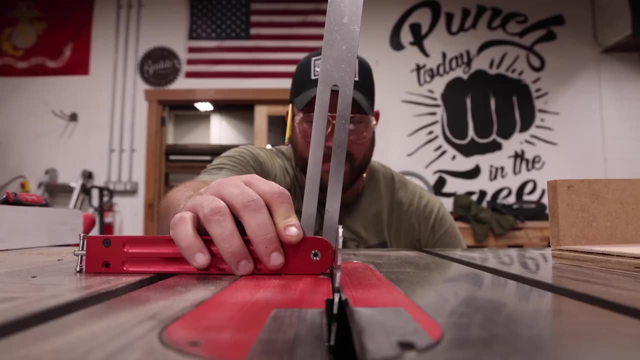 Just under a half hour in, All right. so I'm laying out, I'm going to beena pinboard and I'll transfer those pins and cut those out by hand. All right, so I've got a specialty table saw blade that is angled, that I can cut dovetails on the table saw. 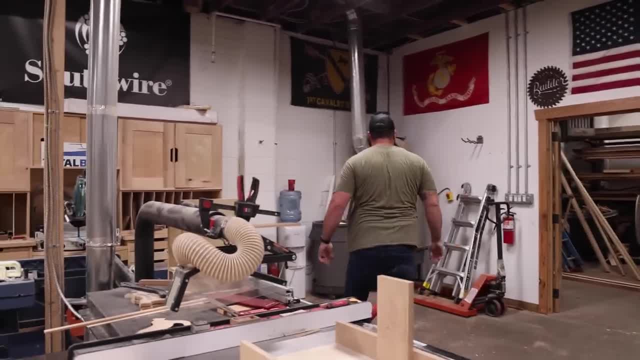 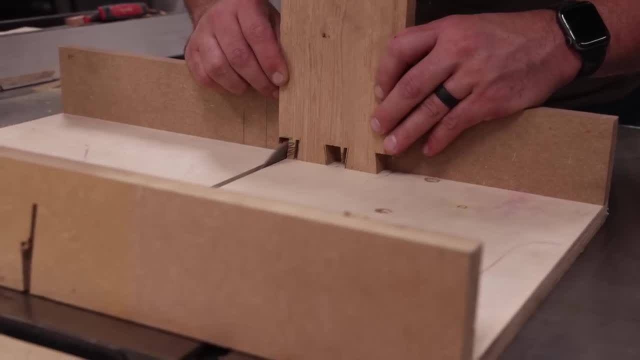 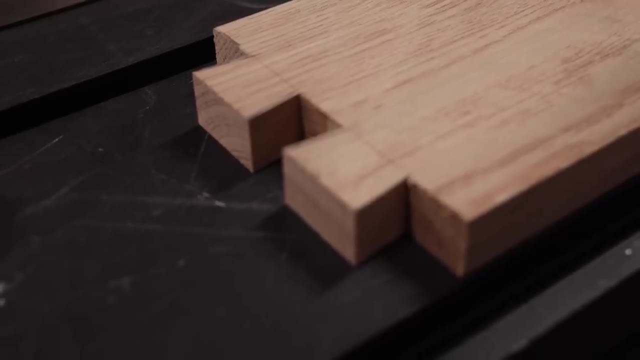 They'll be super crispy and it'll speed things up for me And that does prevent miracles that are just taking me longer than I thought. All right, it's been a minute, so I've been back here. You sure you remember how to do it. 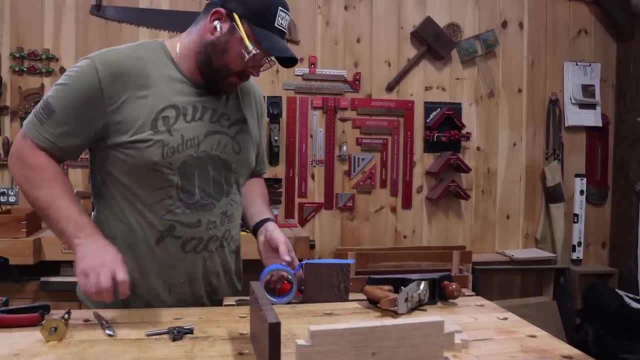 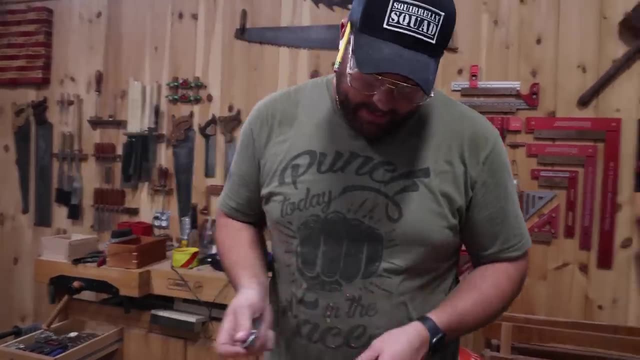 No guarantees. I remember parts enough, but we'll get through it. This is the Mike Pekevich technique for dovetails. He uses this blue tape. The blue tape, especially on this dark wood, gives me an opportunity to really see where my lines. 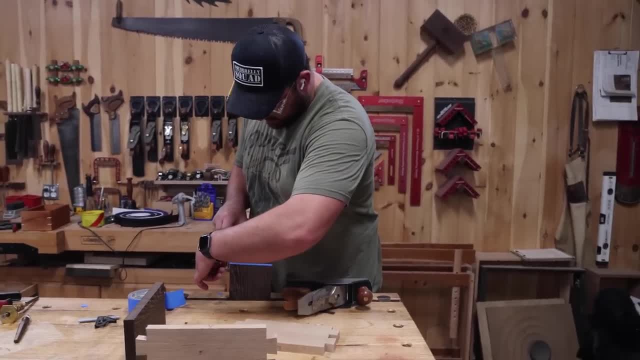 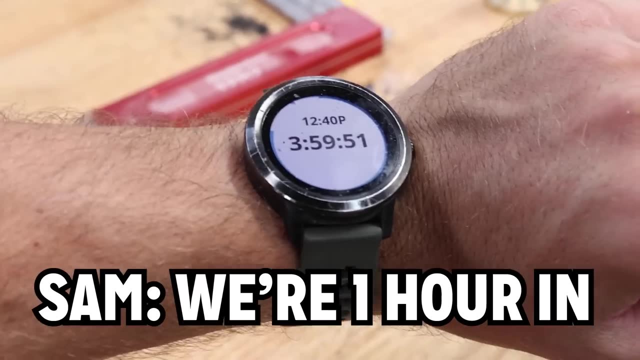 and my cut marks are going to be because I'm going to cut these ones by hand. We're one hour in, So it's going decent. I'm making headway on these. I'm going to use the bandsaw to cut out the waste. 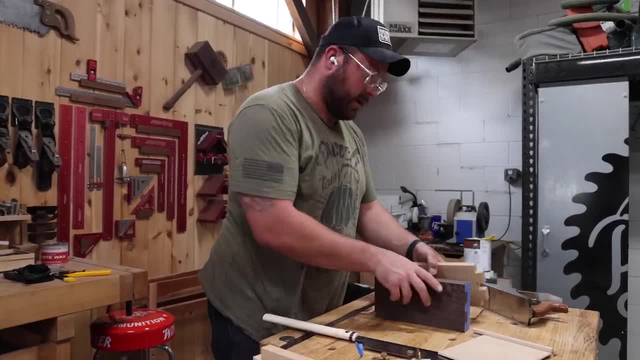 speed that process up a bit. It's just a matter of making sure I keep my parts in the right order, Because that's like when I'm rushing like this, I don't have as much time to like think what I'm doing between each part. 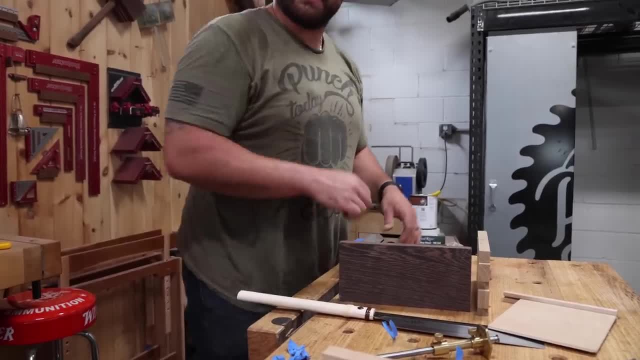 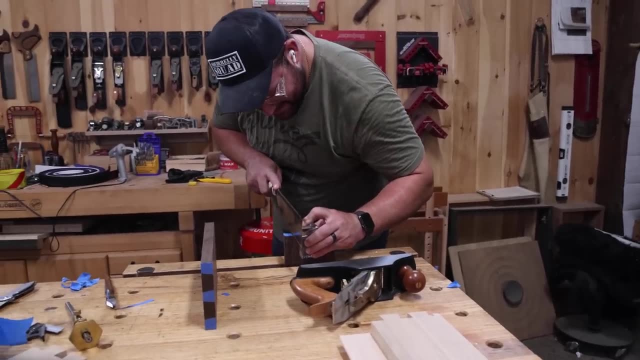 And when you're doing hand, cut anything In one miscut Something that's going to set you back Three hours and 55 minutes. Yeah, dovetails and Sam Green- What do you mean? My dovetails were great. No, you did great dovetails once. 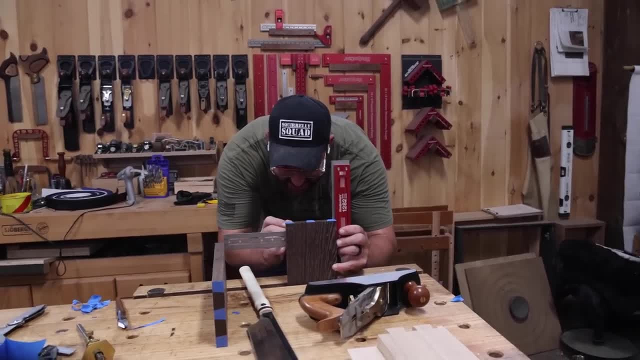 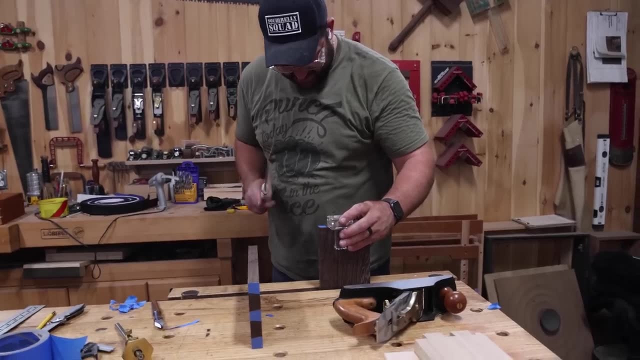 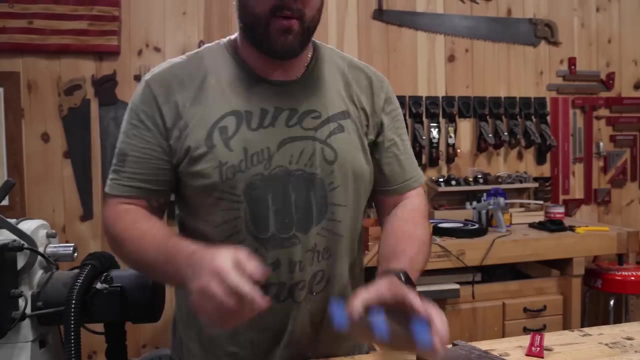 Yeah, around and find out my happy. Actually, didn't you do yours, this exact method? Yeah, explain to me how to do it. And I said: cool, I'm going to just do that. Pretty awesome. So when you do the bandsaw. 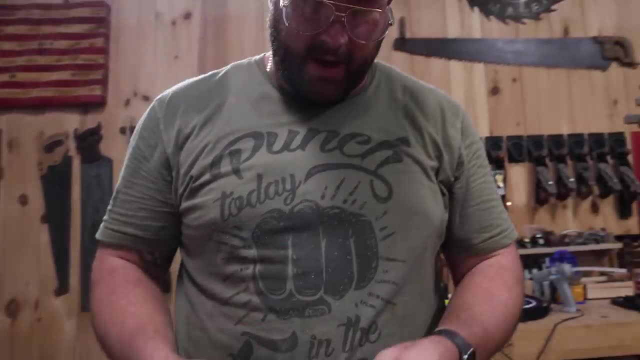 you have to keep the fat parts tall up top, And I think I hurried through it. It should look like this: All of them, And they don't, Which means I'm going to have to re-cut them out, Except this one. 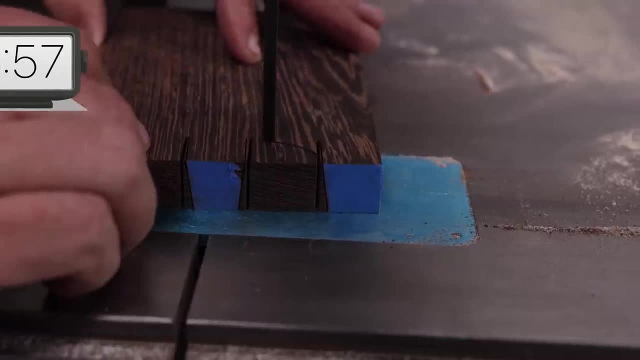 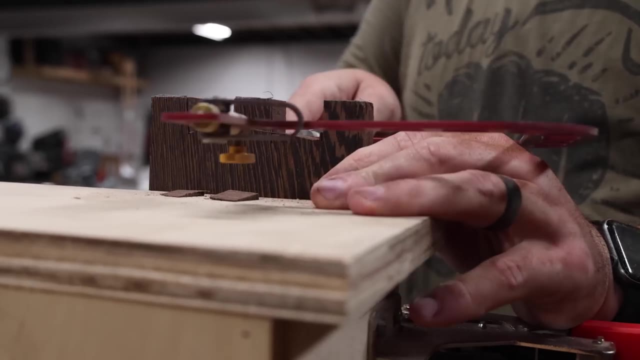 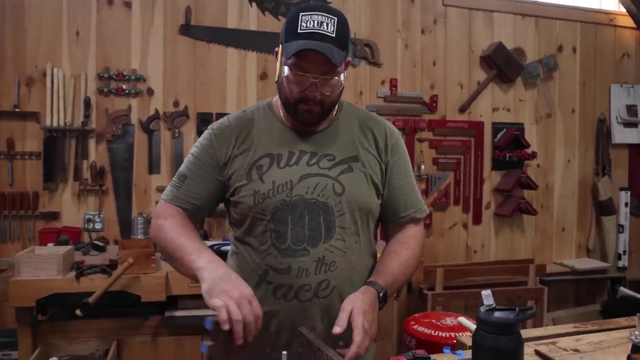 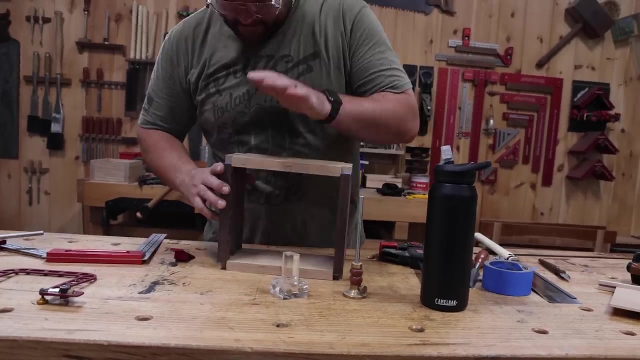 Three hours and 30 minutes. It's working. I don't like this. Are we back to where we were? Closed- 20 minute Detour. We're going to need a little refinement to get everything to fit. Slight bit of sanding. 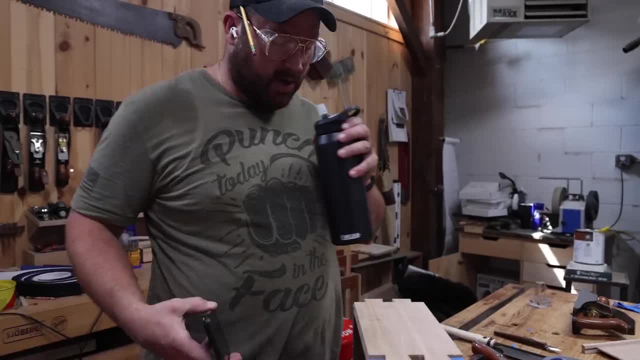 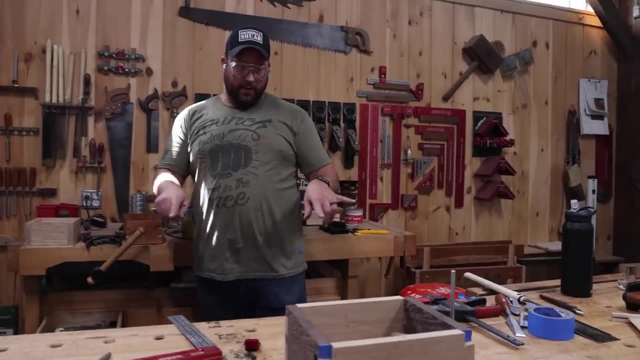 And these should work. Now, Next thing I want to do: this is probably stupid. I kind of was thinking I wanted to do like a foot, Something like that kind of give it a foot and raise it up. Is this a bold move? 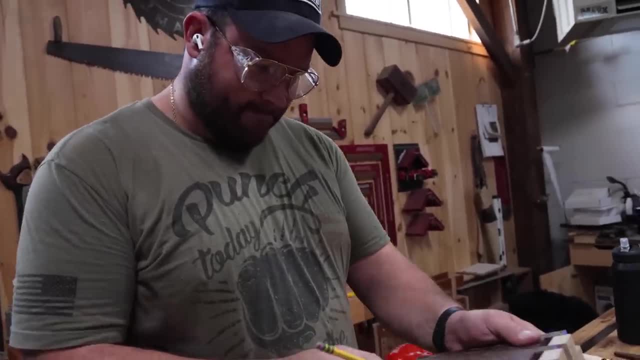 I do believe so, But I mean, you got three hours. what else are you gonna do? you know, Did it break Or did you just bend it? I mean, it's fast. I'm gonna have to check the rule book. 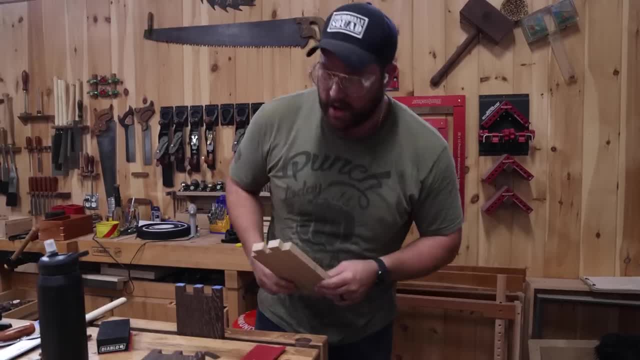 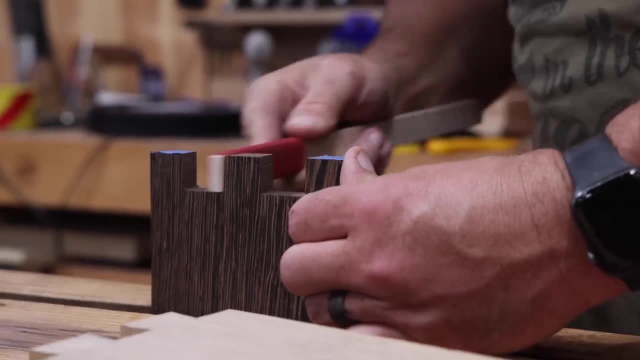 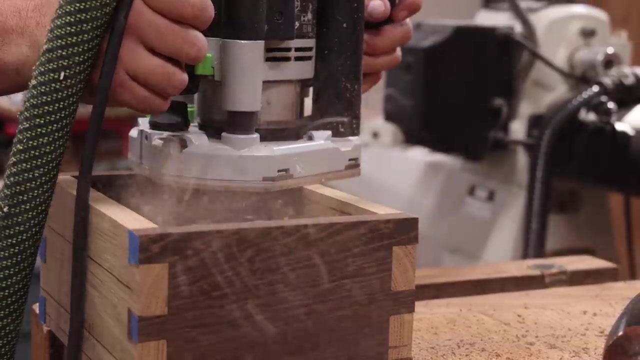 Are we allowed to have maintenance? My employees fix the tools I break. Yes, I do believe it says in the rules. the boss man says: goes, You got three hours. I'm using this technique. I got to cut the lid on the bottom end. 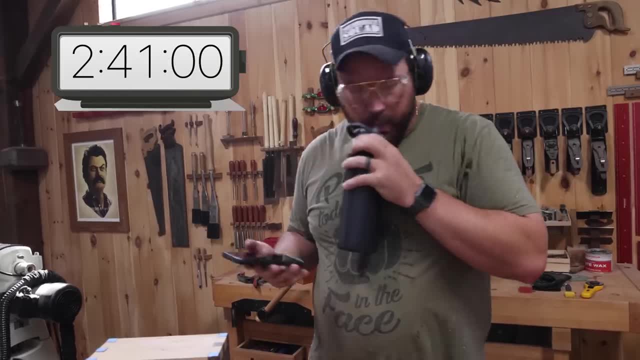 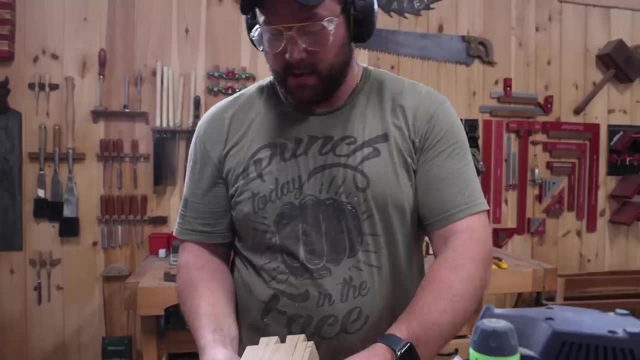 before I glue it up, Look at the bit: Two hours and 41 minutes. Now what I'm gonna do is cut this little detail onto the front bottom of the box, here and here And from there get that thing sanded down. 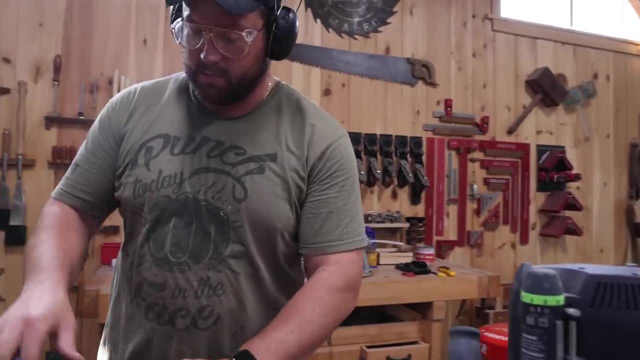 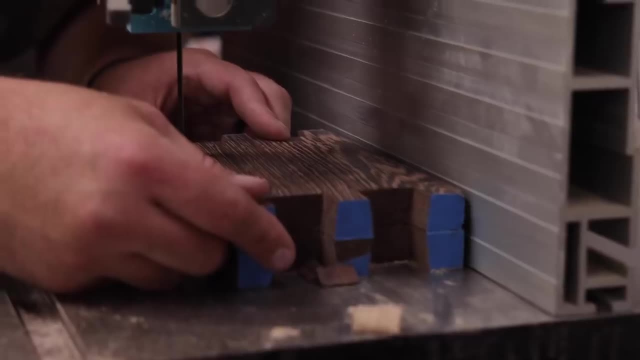 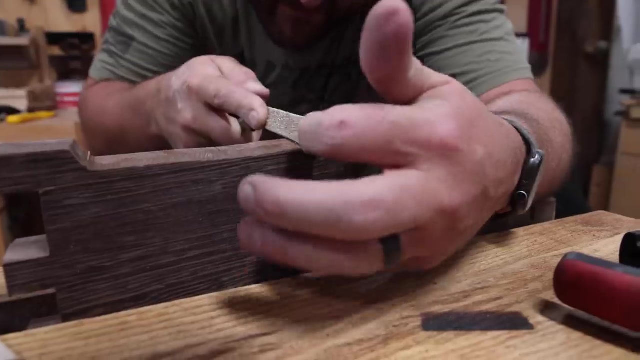 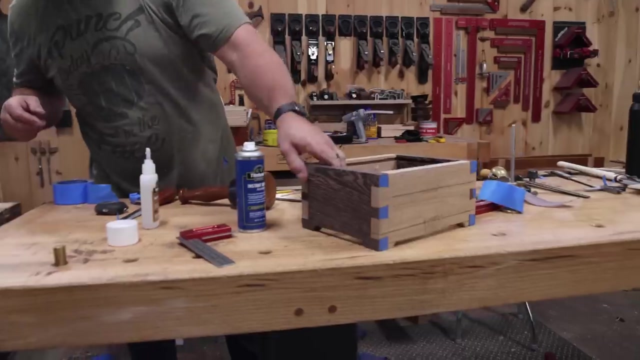 and then work on the lid and the bottom. Once those get in the glue, we're in the homestretch. Have we ever used this? Starting to take shape? That's the general look I was going for with the box, Just those nice little curved feet in the bottom. 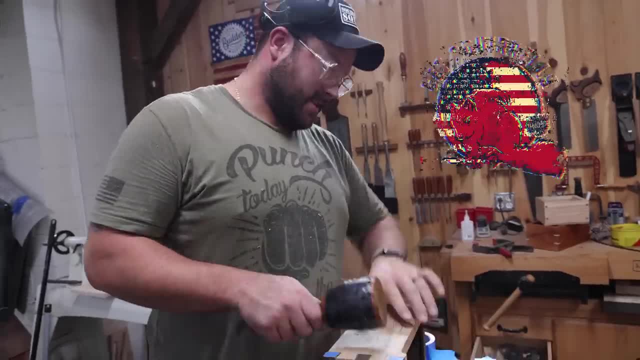 Is that where you thought I was going with it? I wasn't sure what you were doing. I'm just trying to keep up Getting squirrely. What's our time? at My watch died Two hours and 12 minutes. That's gonna be a disappointment if that doesn't fit. 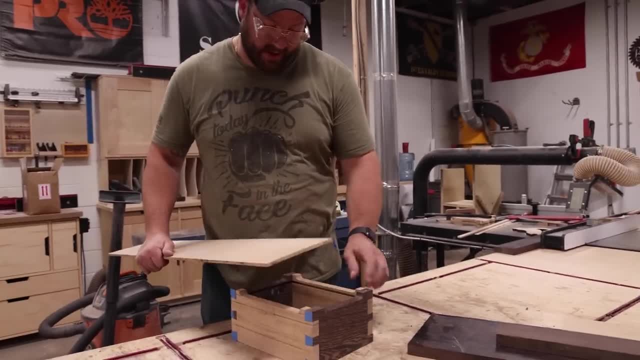 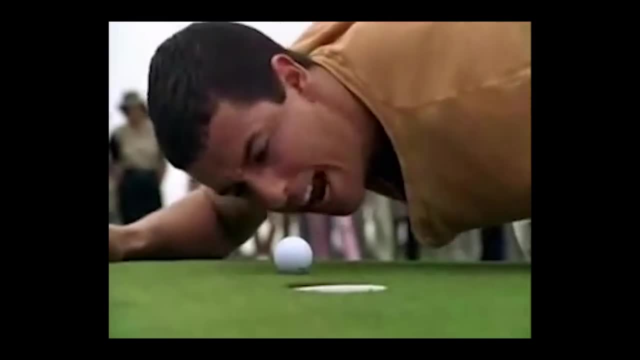 I didn't build it to fit. I was going to use that wider stuff, but I think this fits. Might need a little bit of planing. I'm gonna go to your home. Are you choosing to let me be your home? Damn it. 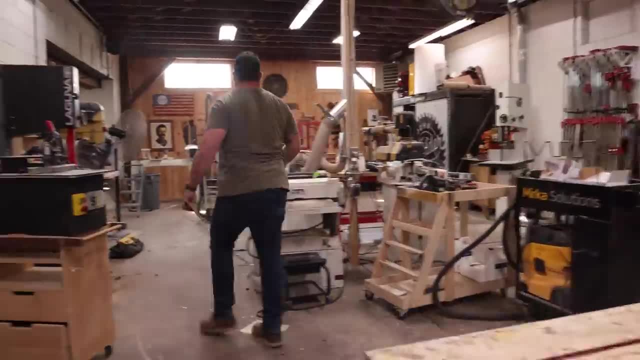 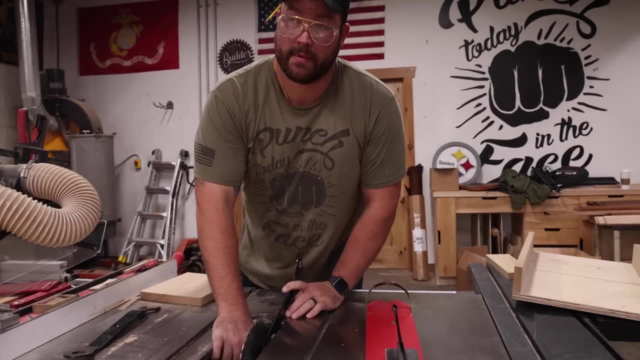 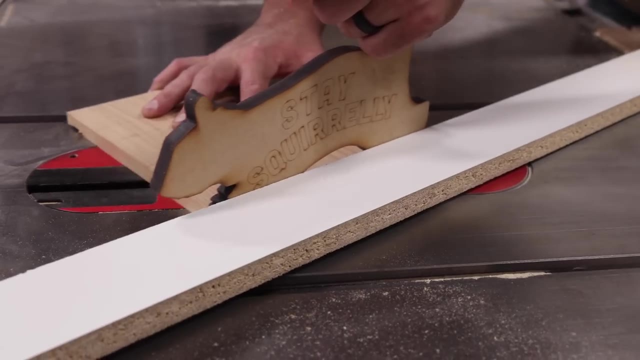 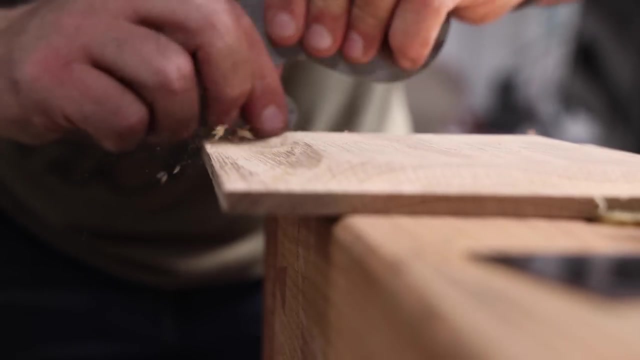 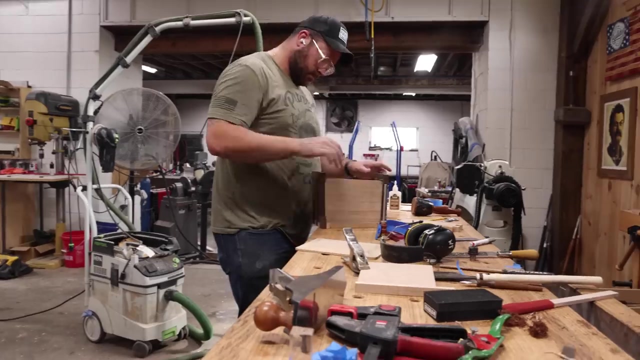 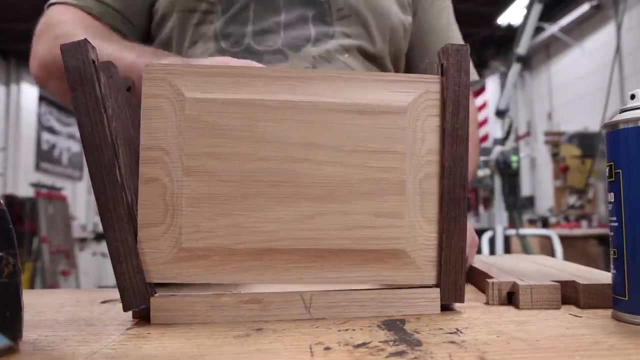 Everything's a hammer. You got two hours. Two, Two, Two. Rip down the box lid, then we're gonna cut coves in the side of the head. Okay, Okay, Here, Here, Here, Here, Here Here. 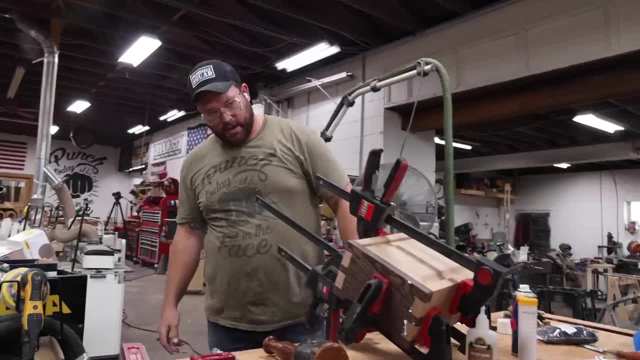 All right, Okay, Cool, All right, Just trying to use what I have. get a water and let's make a handle. I'm going to have to keep it basic because I don't have time. There it is. That's what's speaking to me. 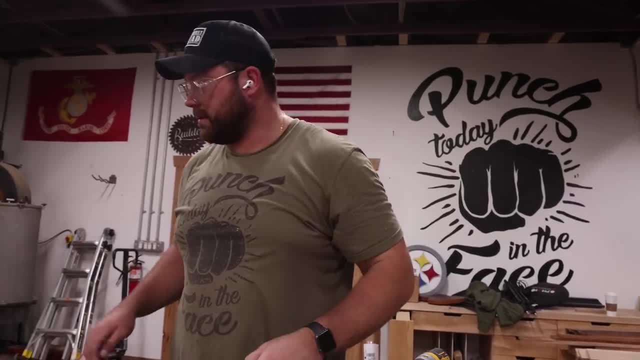 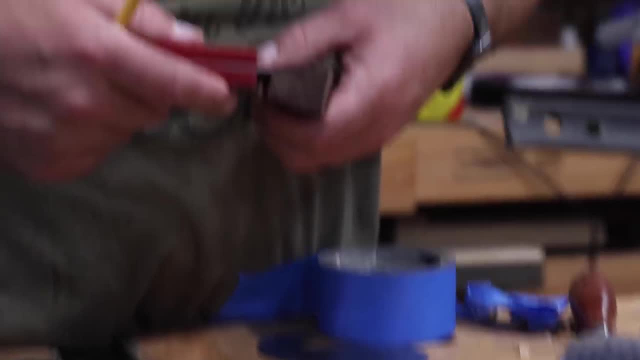 Curve and the part I'm going to cut out: One hour three minutes and five seconds, And that is Jordan. Yeah, This can't hold this ridiculous mess I made All right. That's it, guys. All right, Cool. 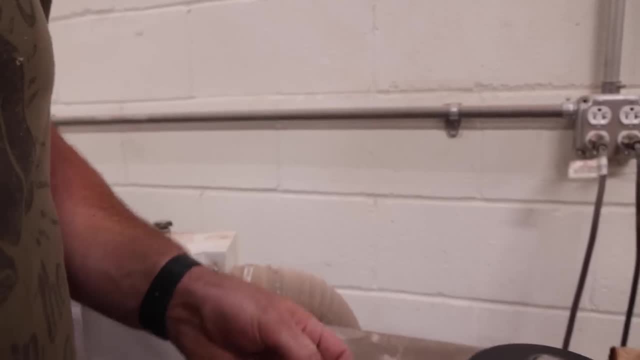 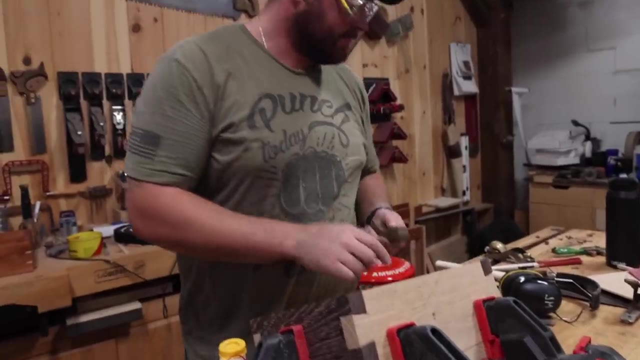 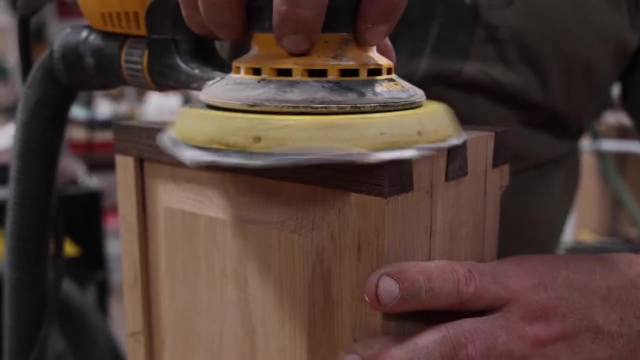 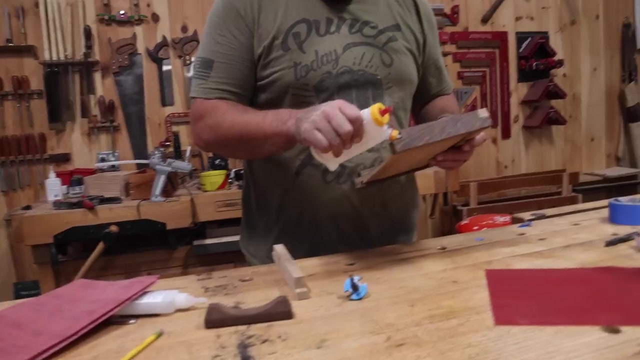 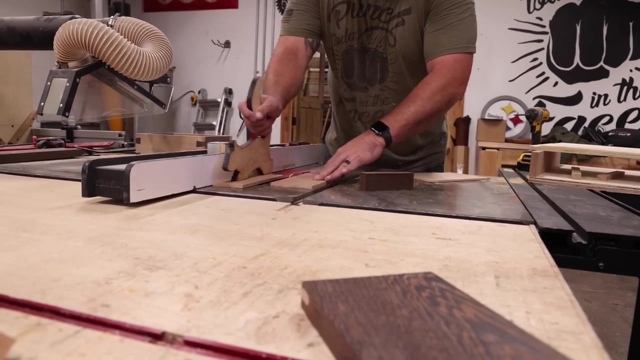 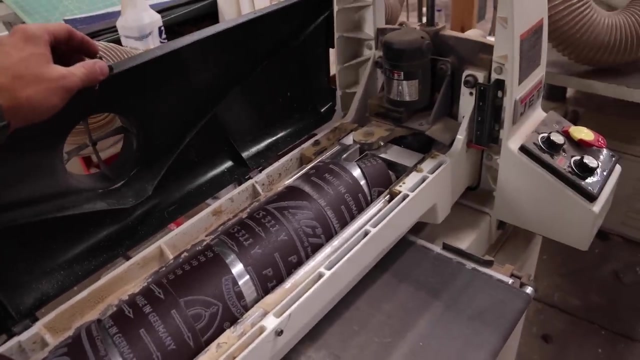 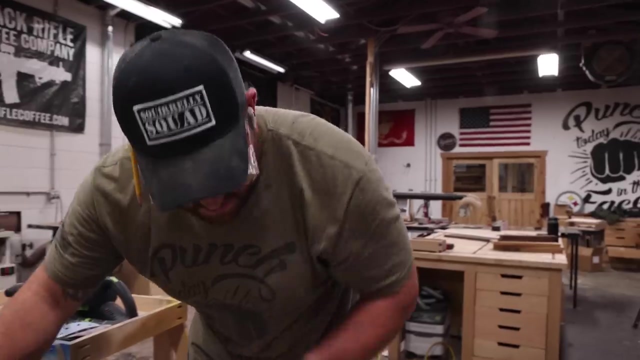 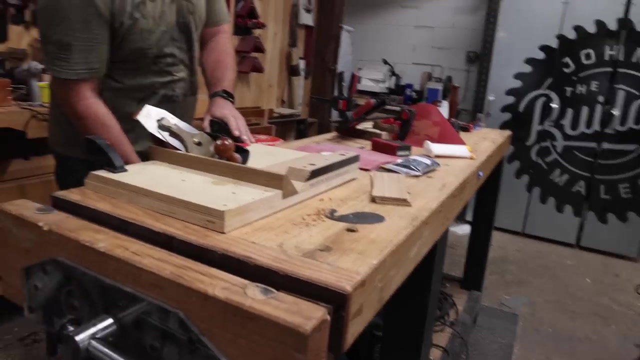 One hour. We think. Samwise, It's a box. hey, it's gonna be pretty cool. I think I don't know why we're approaching this like a challenge: make shitty stuff. I Not good. Can you put a new belt on that? please Forget how to do this. 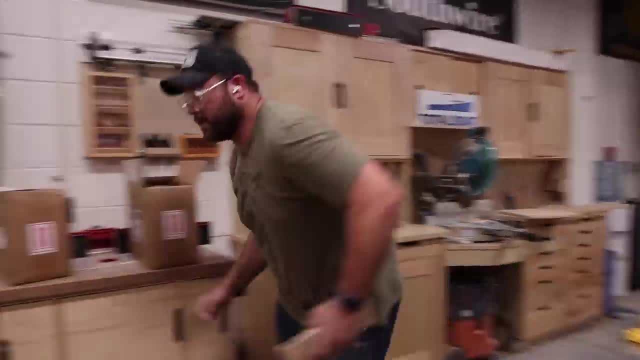 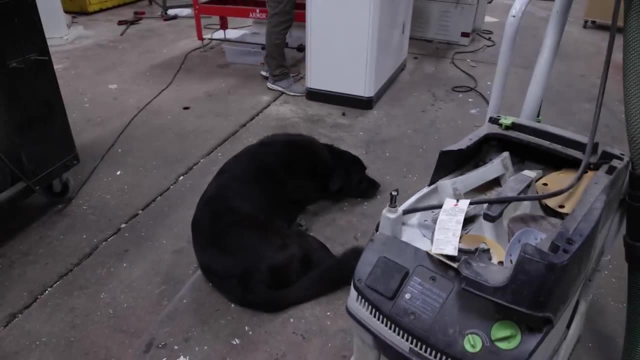 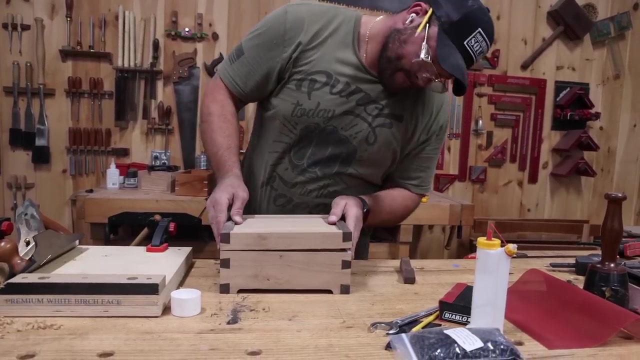 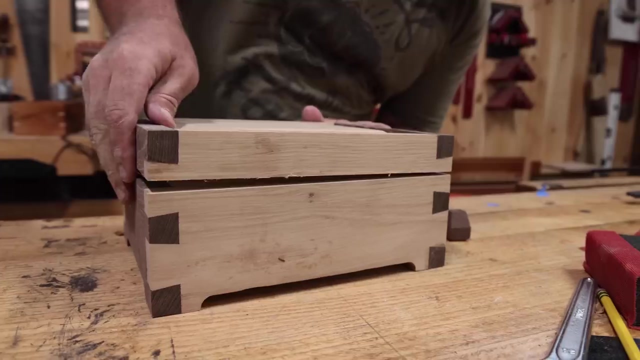 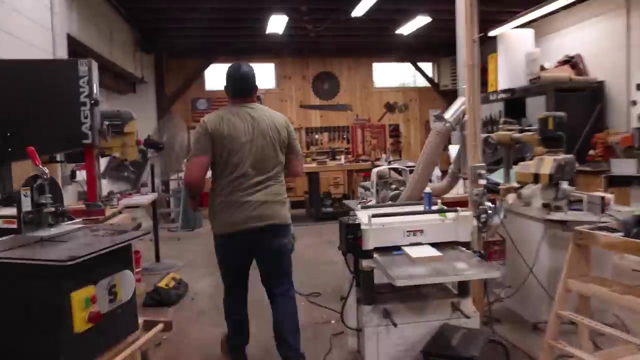 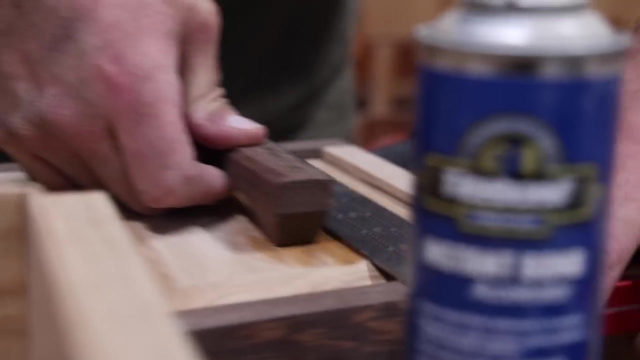 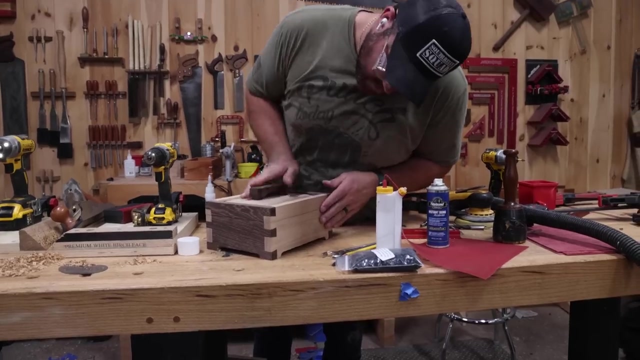 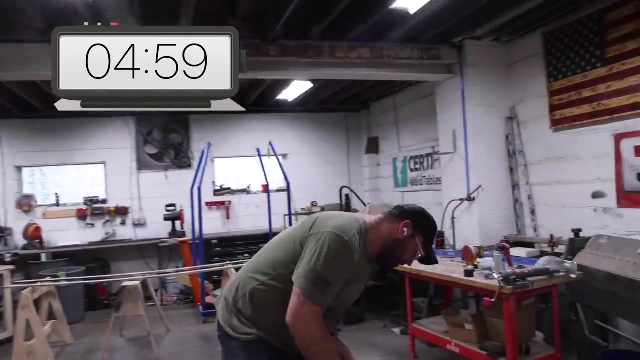 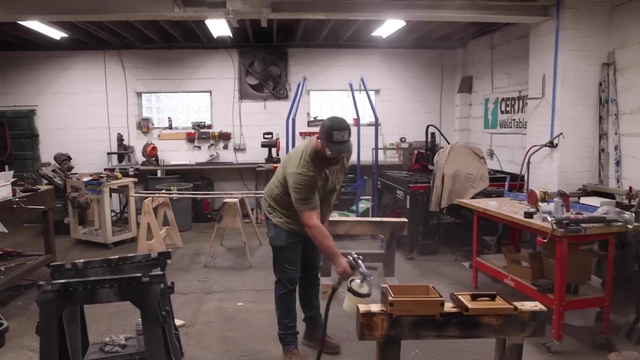 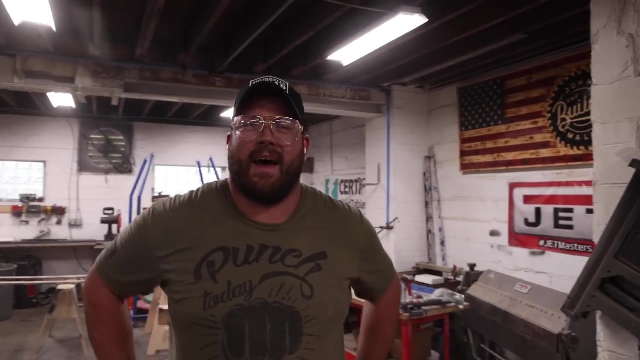 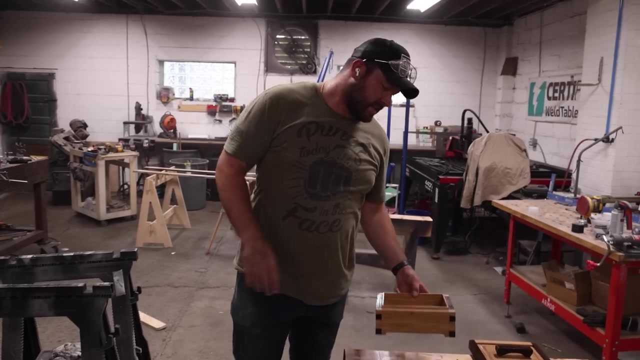 You 16 minutes looks really good. I'm very surprised What I'm? Where's my fucking one? screw. You have six minutes. You got five minutes. My back hurts four minutes to stay. So we will argue the inside and bottom aren't finished technically. the challenge was: can I get it done, cuz I mean like yeah.